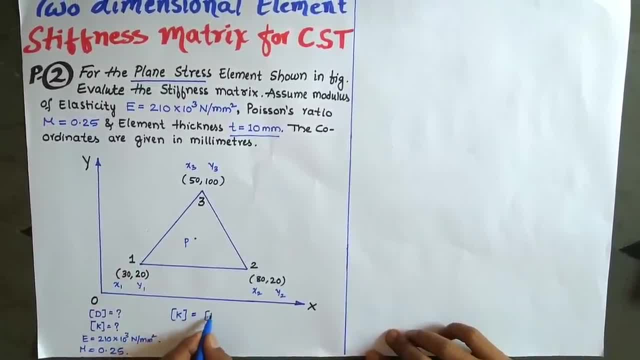 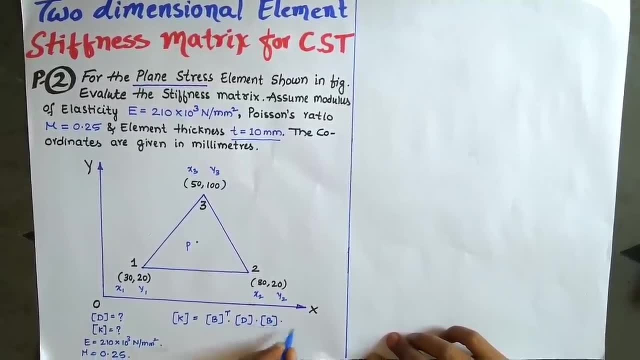 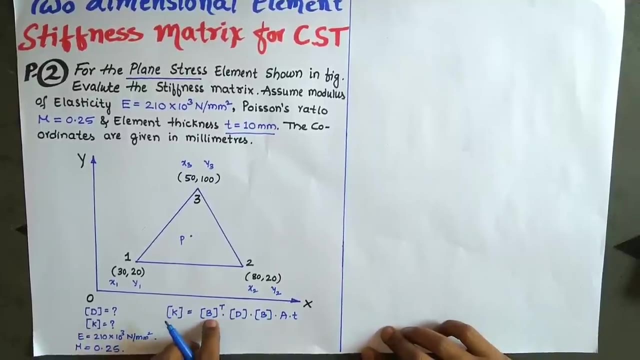 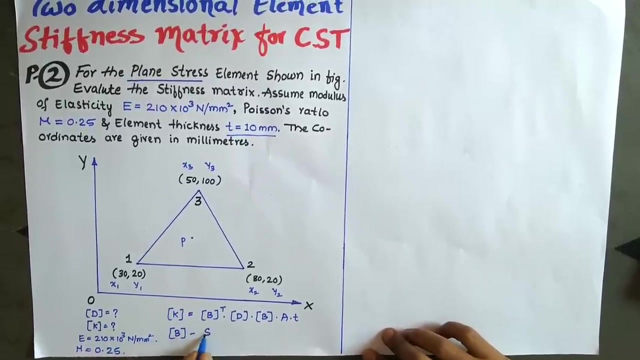 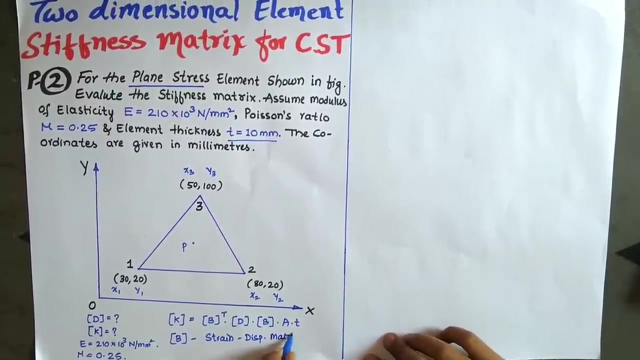 for the triangular element it will be b, transpose into d, into b, into a, into t. so this is the equation to calculate the stiffness matrix. so where b matrix it is called strain and displacement matrix. where b matrix it will be strain displacement matrix, where d it will be stress strain displacement. 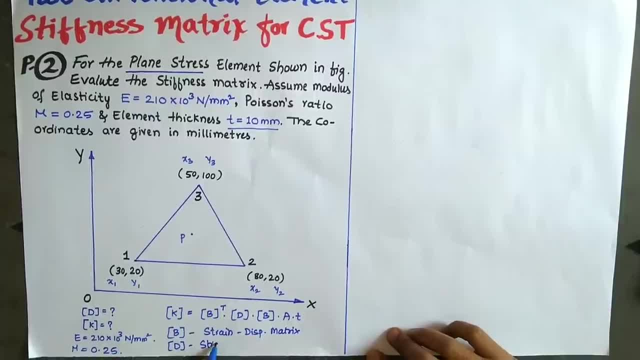 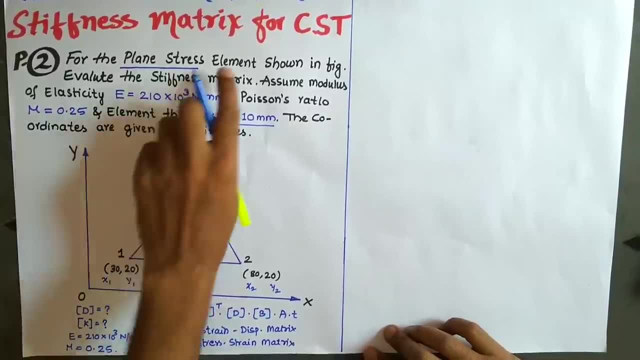 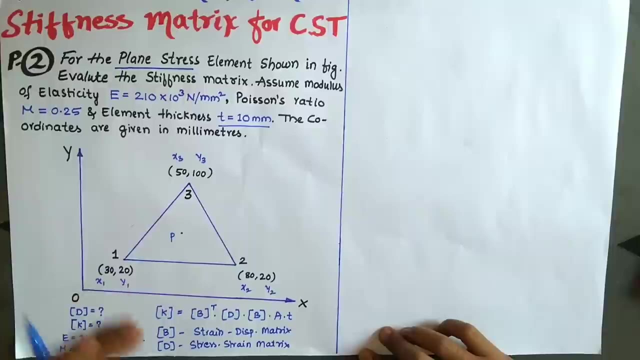 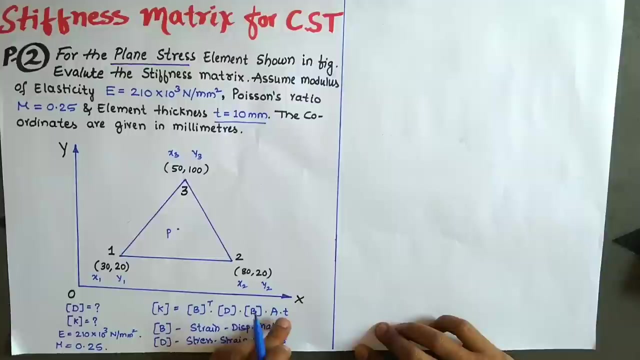 matrix relation between stress strain. so this will be changed based on the type of element. so it is plane stress. for plane stress we have the thickness matrix. if it is in plane 10, we will have the another matrix equation. okay, and again, a, it is a area of the element and t is the thickness of the element. so we will calculate one by one now. 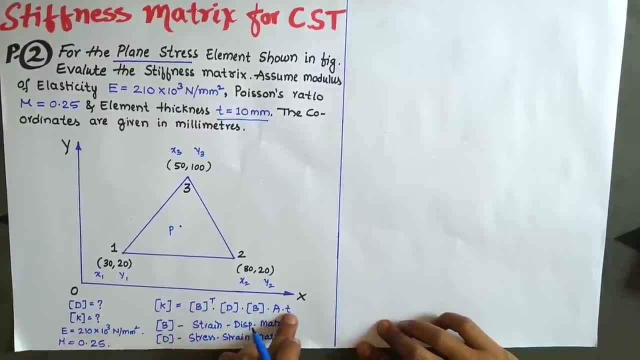 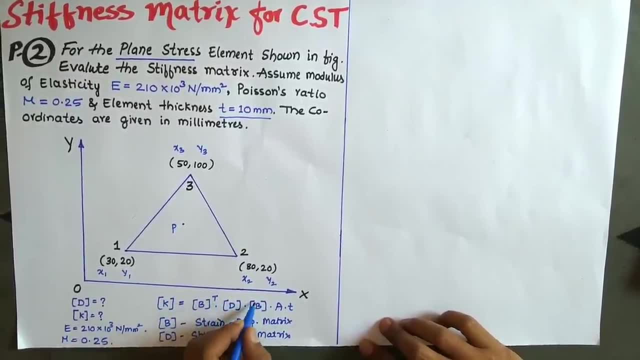 first we will calculate the area and next we will calculate the thickness, then we will calculate the d matrix and then we will calculate the b matrix. so, b, once you calculate the b matrix, we will make the transpose of the b matrix, so we will重 wood to the value of b matrix and then database sådan. matrix done and then we will call div matrix- is needed if the –or the matrix that we use for that, we will call the g matrix. so it is b which will be b transpose to the b matrix. so every step will be b 표. then in listen what you can calculate sharp, extent them, enforcement, every step could. 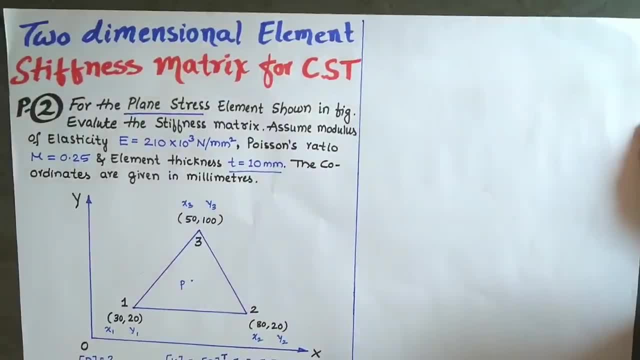 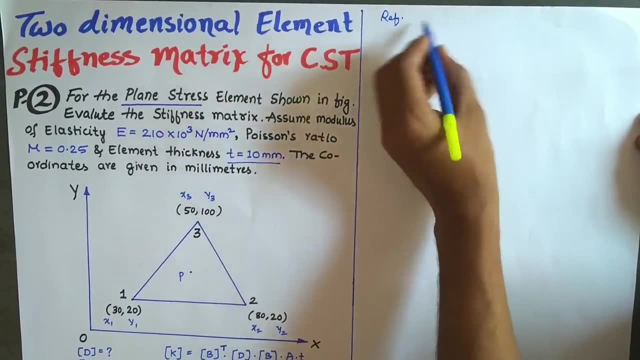 it be any matrix, random space, so that will be dynamic. first suppose something will be W, so according, get b, transpose. okay, so now from the referring of the given diagram, given element, we will calculate the coordinate system which are already mentioned here. x1, y1- we have to write separately referring. 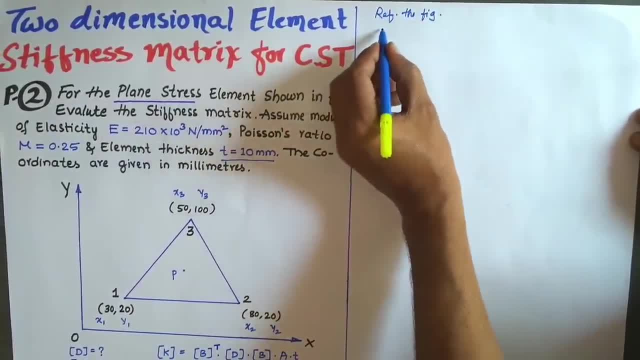 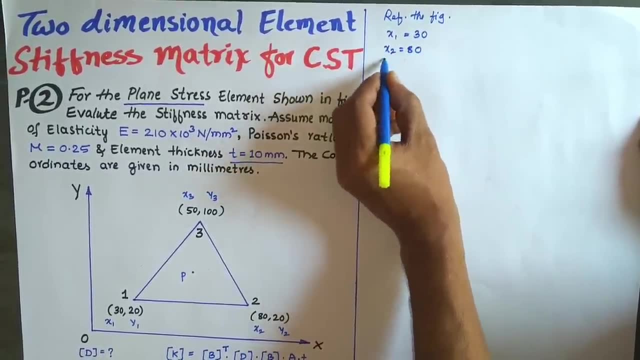 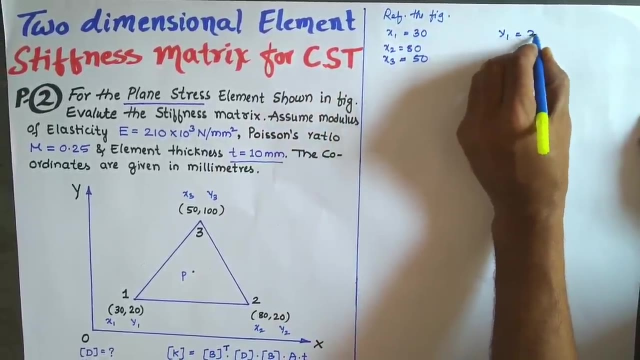 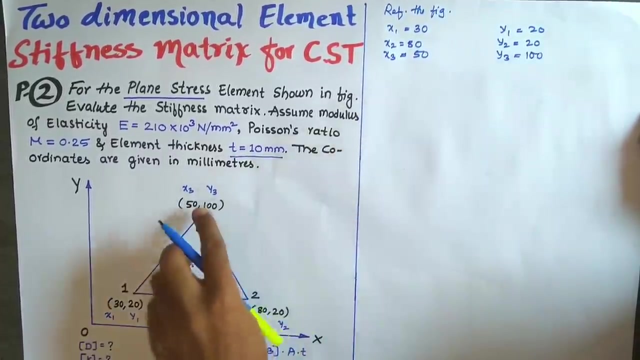 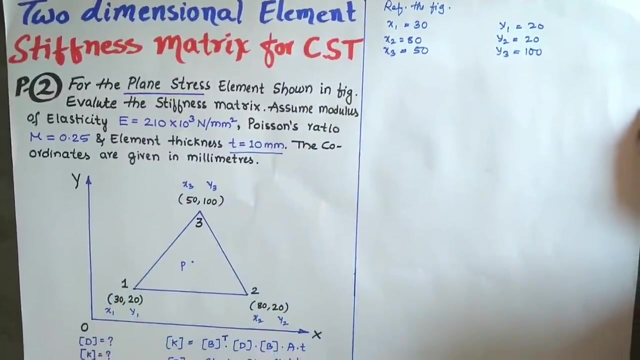 the figure. so x1 is 30 and x2 is 80, x3 is 50. similarly, y1 is 20, y2 is 20 and y3 is 100. okay, so these coordinates i have written separately. so after that the, the i have already written, and all are in millimeter. the standard unit of the given problem is in. 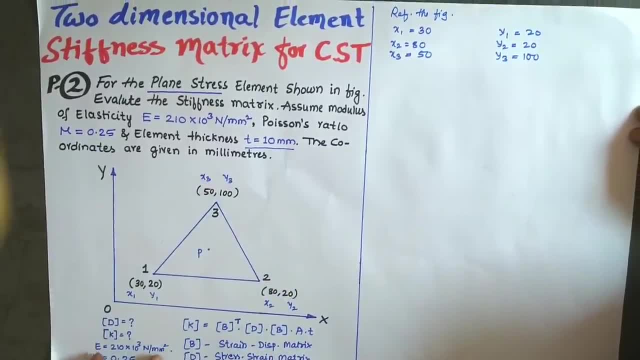 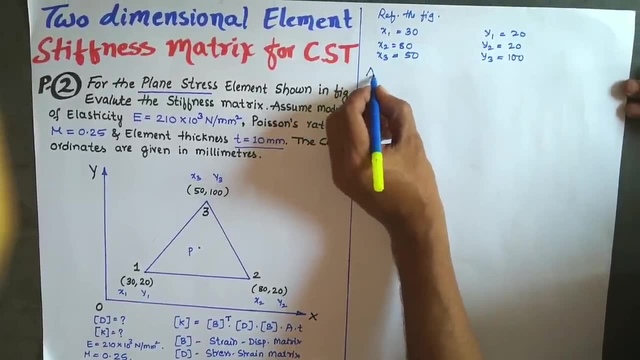 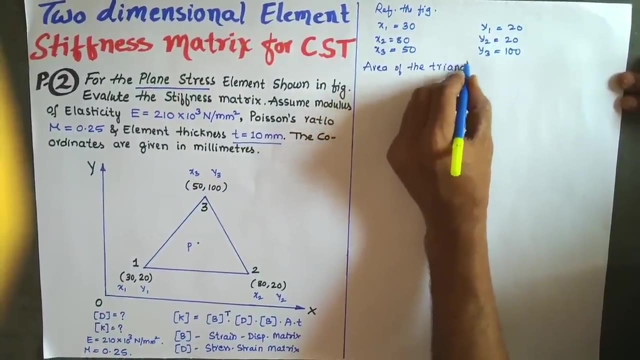 millimeter, so coordinates also in millimeter and the material property is also in millimeter: newton per millimeter square. okay, so after that we will calculate the area of the triangle. so area of the triangle where a is equal to. area of the triangle where a is equal to. 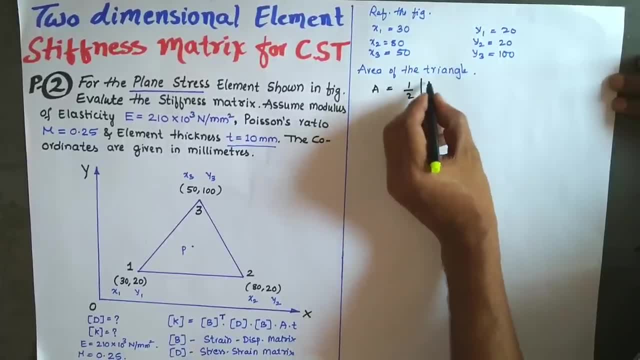 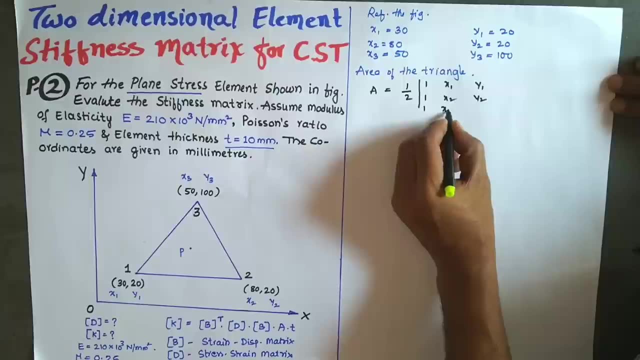 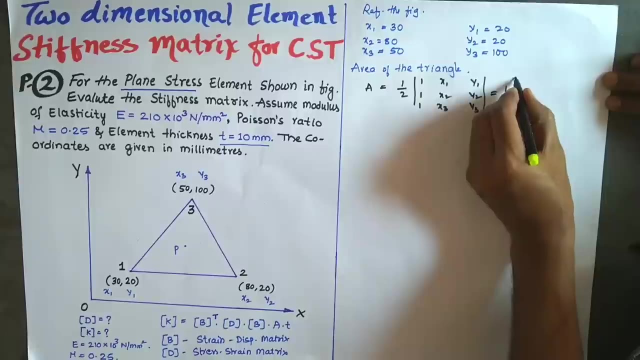 area of the triangle where a is equal to half determinant of 1 x1, y1, 1 x, 2, y2, 1, x3, y3, 1x3.. okay, so one by two. x1, y2, 1x3, y3. okay, so one by two. 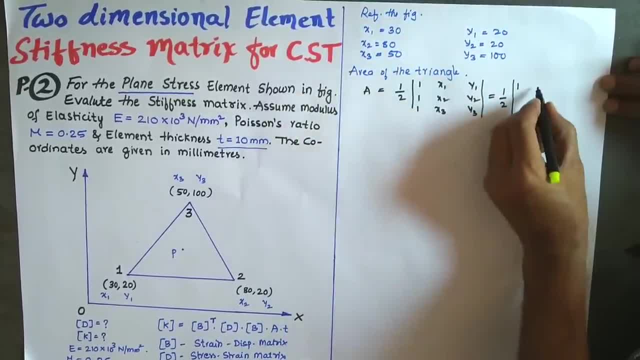 X2 and y. so x1 is 30, y, 1 is 20, Yap, reversed solvent: 1, x2, h2, y2 is 80, 0, x1, y1, x2 is 30, y1, x2, h0, y1, x, 2, h0, x2, y2, 1, x3, y3, 1, x2, h1, x1, h0, h0, x2, h0. so x1 is thirty one, x2, y1, x2, y3, y1, six, three, y3. ok, so 1, x2, eeg, 3. okay. so 1 by two. substitute the value of x, x and y. so x one is 30, y, 1 is 20, similarly one. x2 is 80, y, 2 is 20, x, 1 is 30, y, 1 is 20. similarly 1, x2 is 80, y2 is 20. 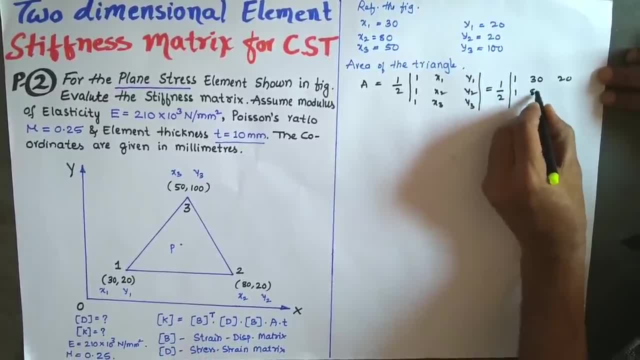 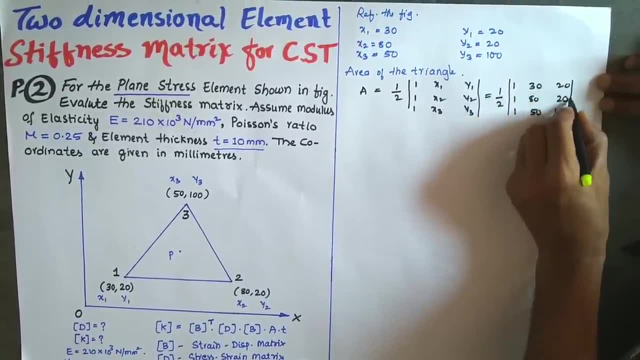 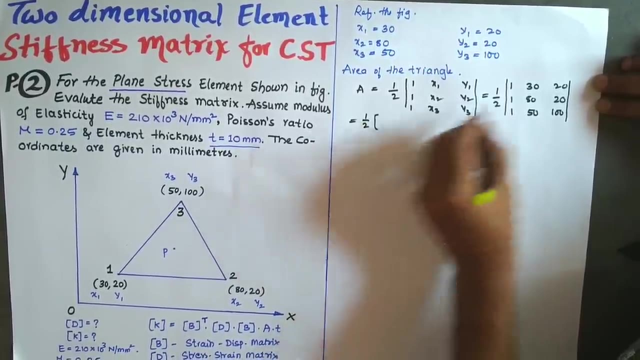 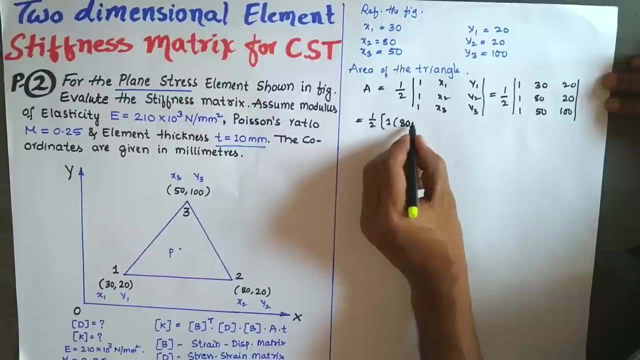 Similarly, 1x2 is 80, y2 is 20, 1x3 is 50, y3 is 100.. So 1 by 2, keep it as outside Now. so 1 in the bracket 80 into 100, so 8000, minus 50 into 20,, so 1000. 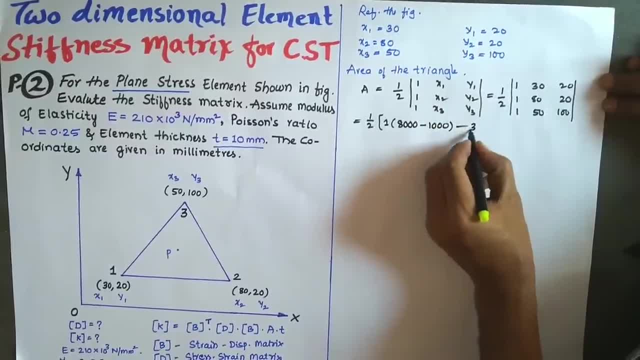 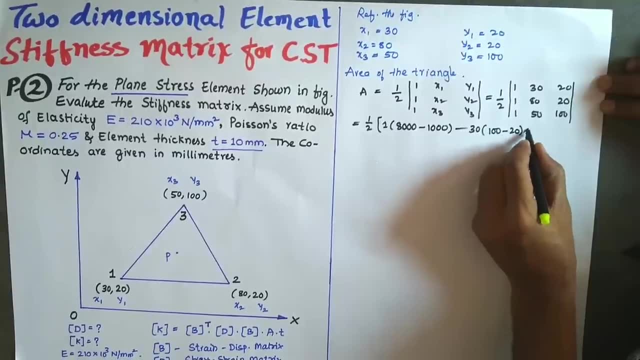 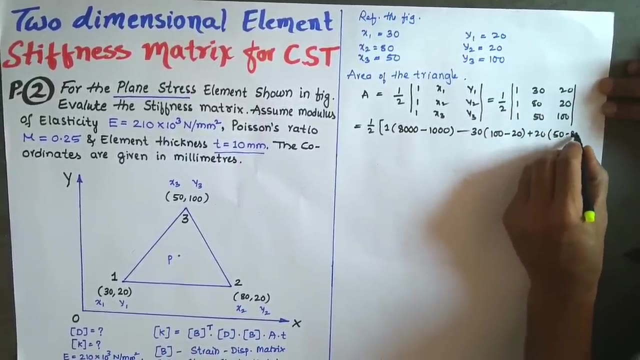 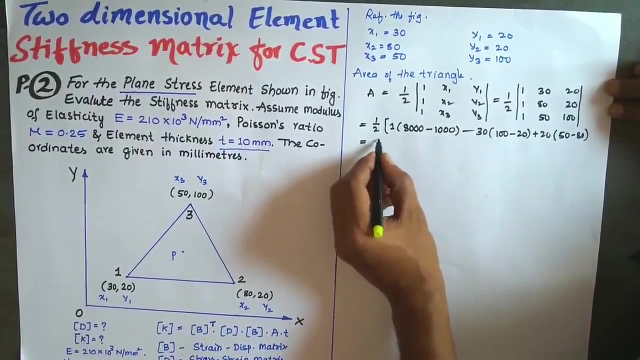 Again minus 30,, so 100 minus 20, plus 20 for the third row, So 50 minus 80,, 50 minus 80. So we get, after calculation, 1 by 2, so 8000 minus 1000, so 7000.. 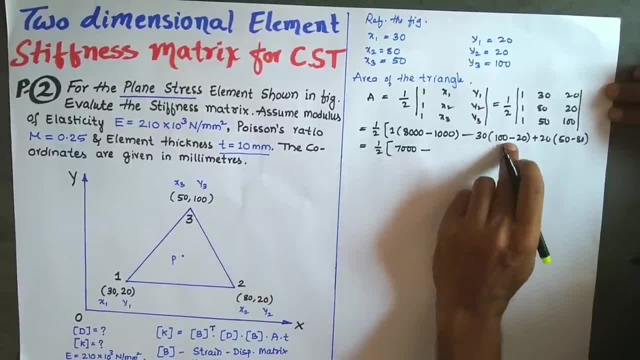 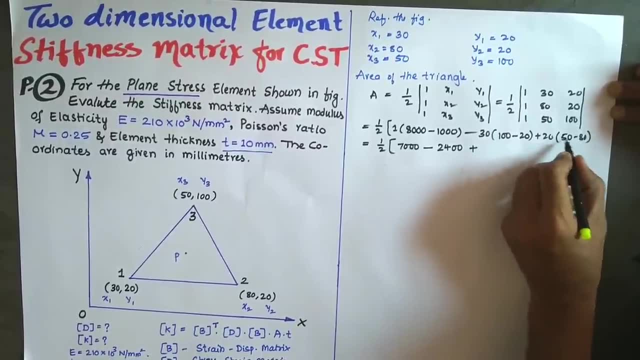 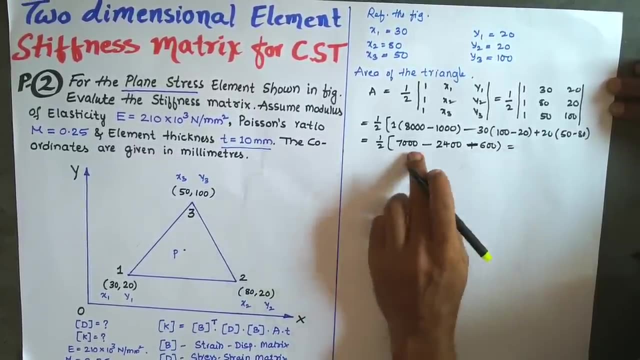 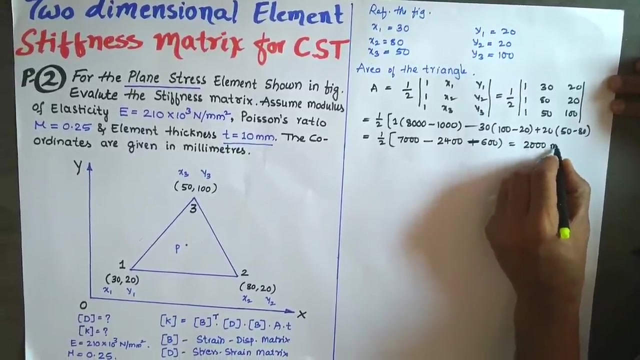 Minus 30 into 80, so it is 2400, plus, here it will be minus 30 into 20, so you will get minus 600.. So this is a minus 600.. Okay, so now, after making calculation, we will obtain 2000. millimeter square is the area for the triangular element. 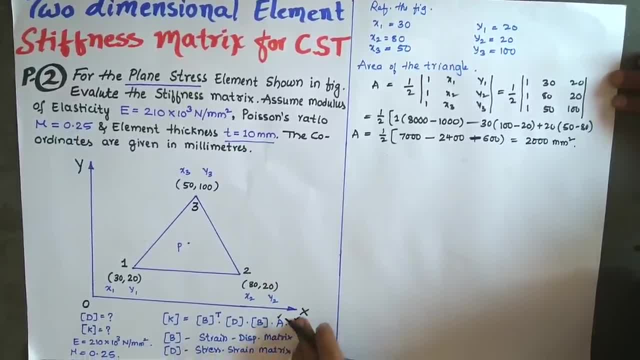 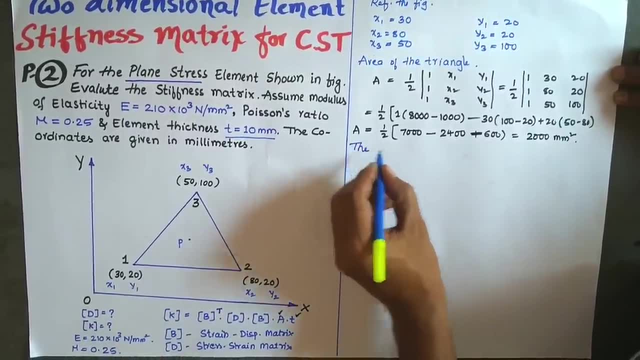 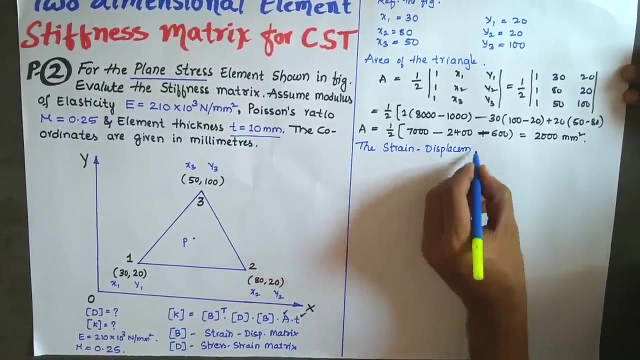 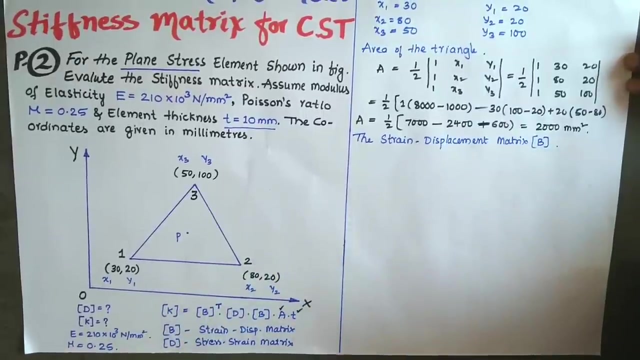 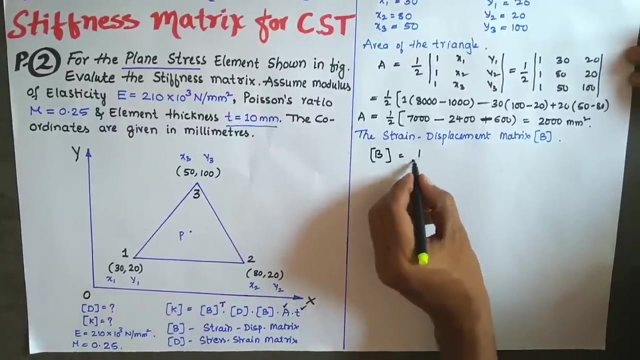 So we obtain area. Now we have the thickness also 10 mm. After that we will calculate the B matrix first, The strain displacement matrix. So that will denote with B. The equation for the B matrix is 1 by 2a. a is the area. 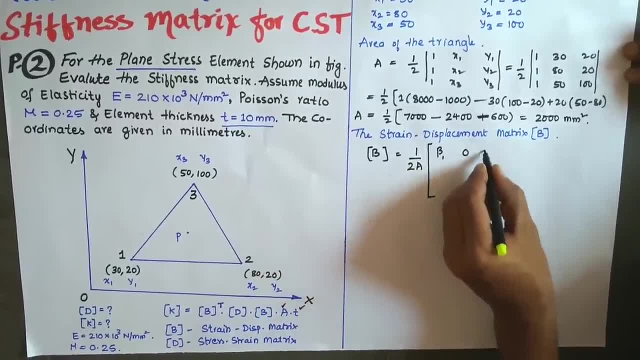 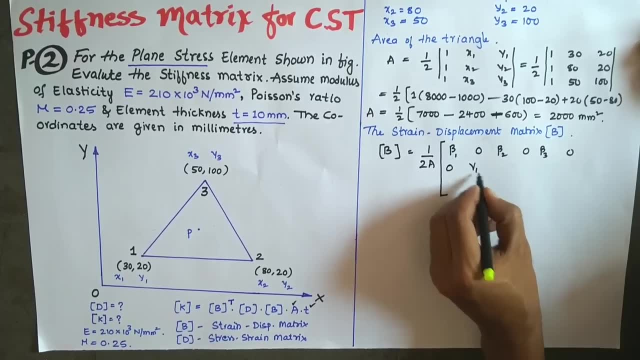 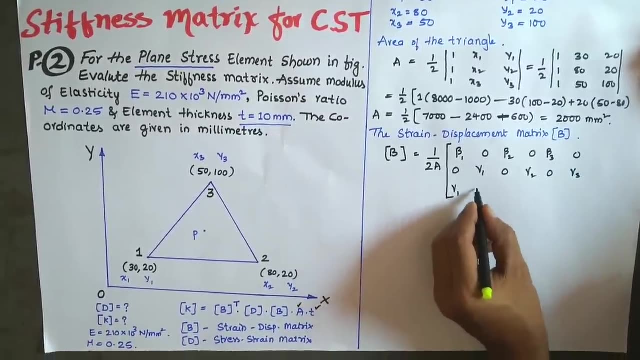 So here: beta 1, 0, beta 2, 0, beta 3, 0.. Next, 0, gamma 1, 0, gamma 2, 0, gamma 3.. Now gamma 1, beta 1, gamma 2, beta 2, gamma 3,, beta 3.. 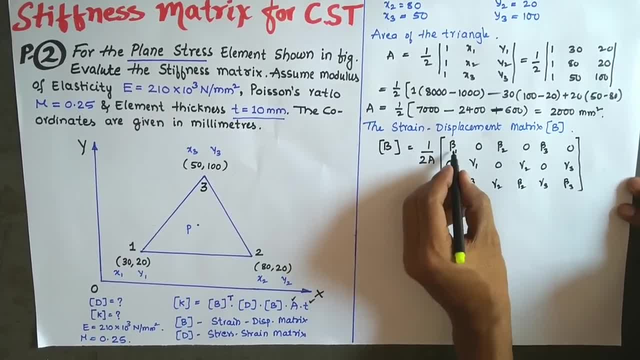 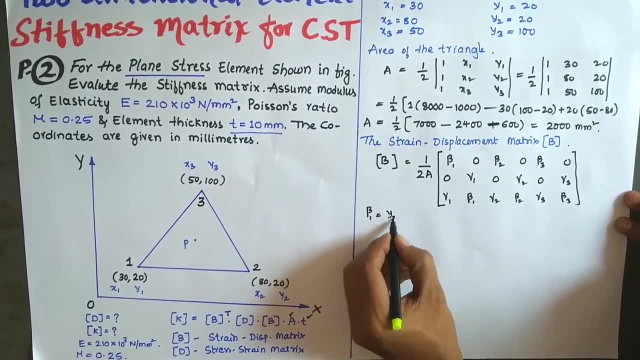 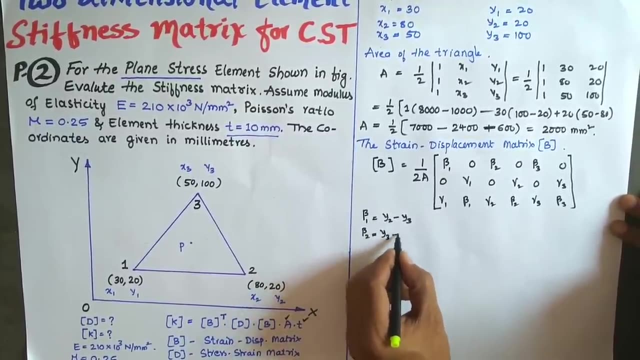 Okay, now we will know what is beta and what is gamma. So beta 1 is nothing, but it is y2 minus y3.. Next, beta 2, y3 minus y1,. beta 3, y1 minus y2.. 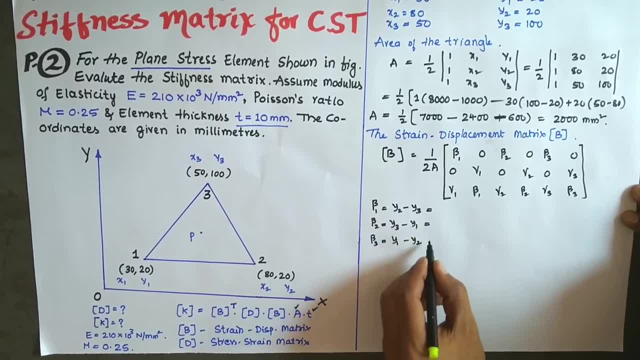 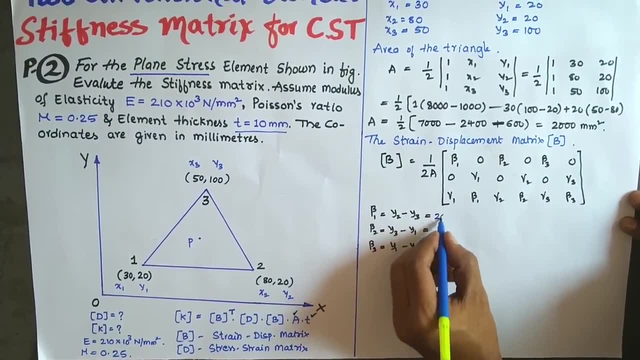 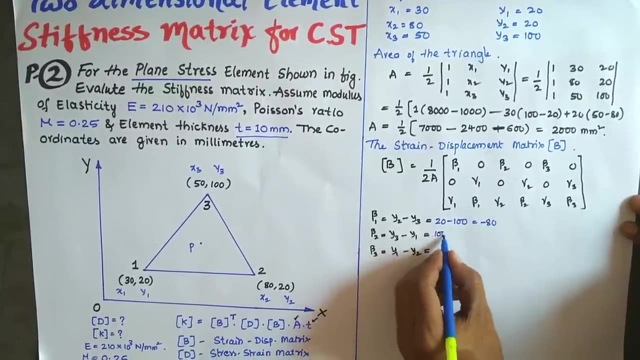 Okay, so we will calculate first beta value, So beta 1.. So y2.. So beta 1 is 20 minus 100.. 20 minus 100.. So we got minus 80.. Similarly, y3 is 100 minus 20, y1.. 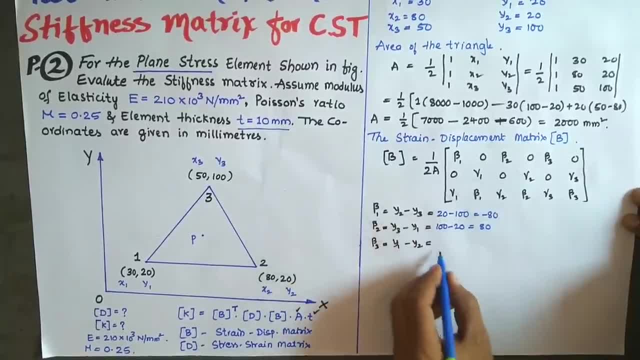 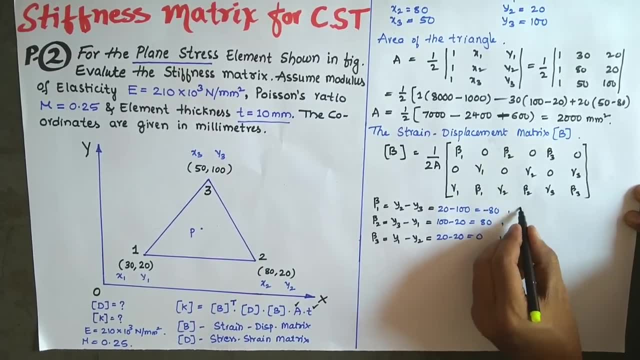 So plus 80.. So y1 minus y2, 20 minus 20.. So it is equal to 0.. Okay, So now we will calculate gamma 1.. Gamma 1 is equal to x3 minus x2, gamma 2.. 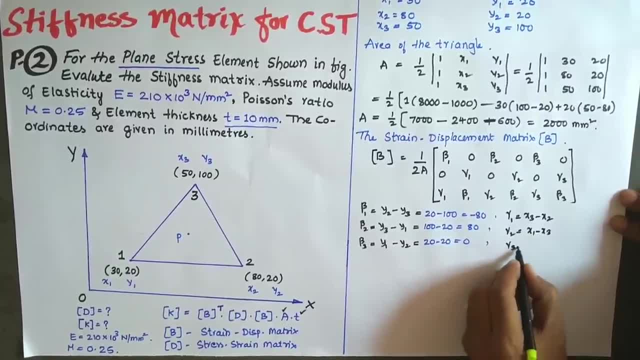 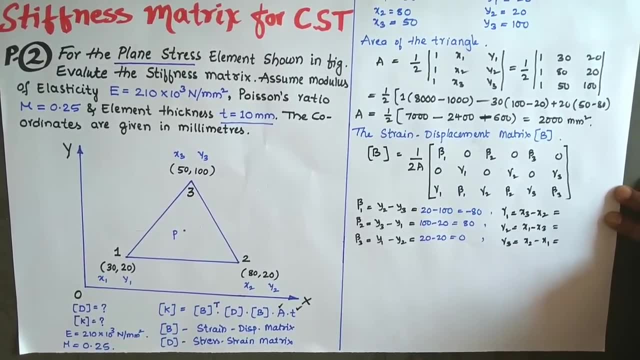 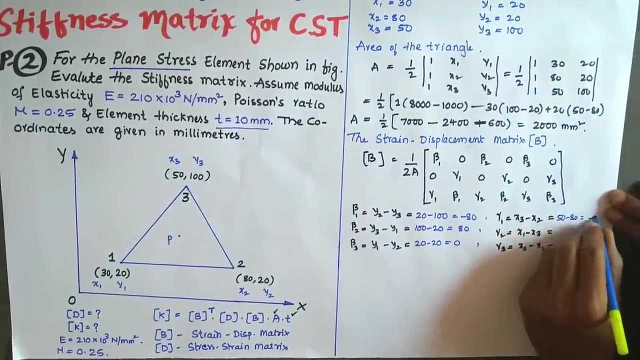 x3 minus x2, gamma 2.. x1 minus x3, gamma 3, x2 minus x1.. Substitute the x value in this, So x3 is 50 minus 80.. So we obtain minus 30.. 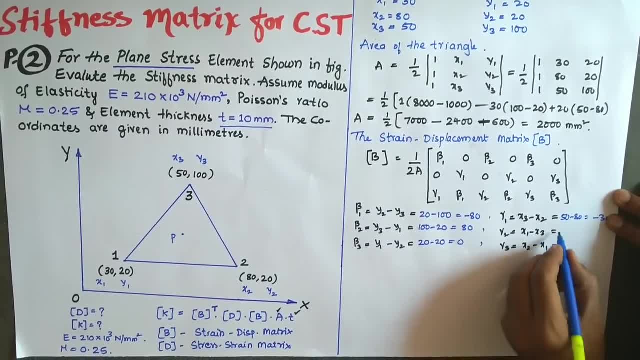 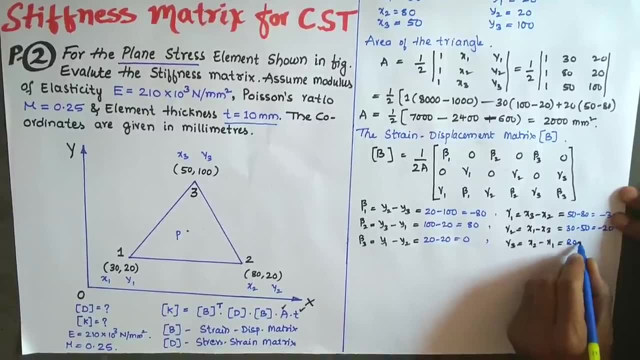 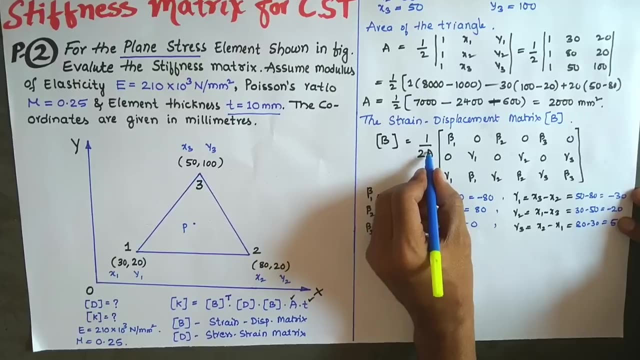 x1 minus x3,, 30 minus 50. So it is minus 20.. x2 minus x1,, 80 minus 30. So it is 50 is the value. So we got all And also we obtained the area for the triangular element also. 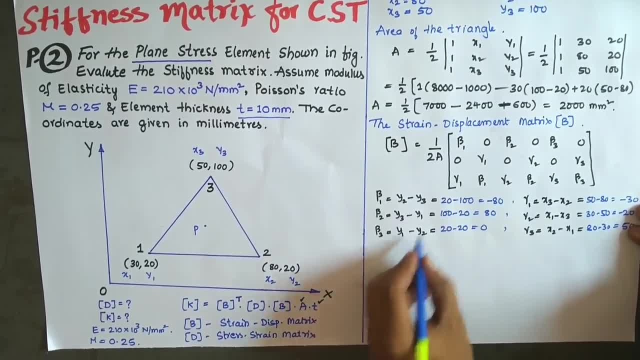 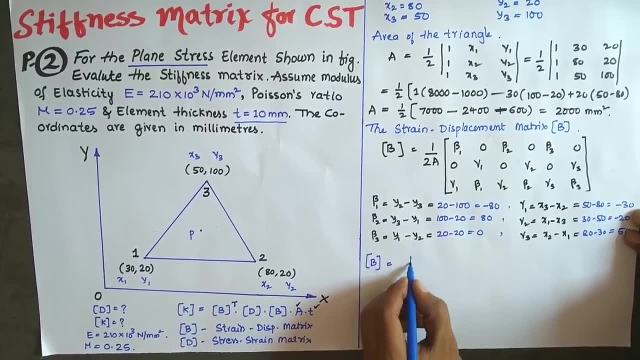 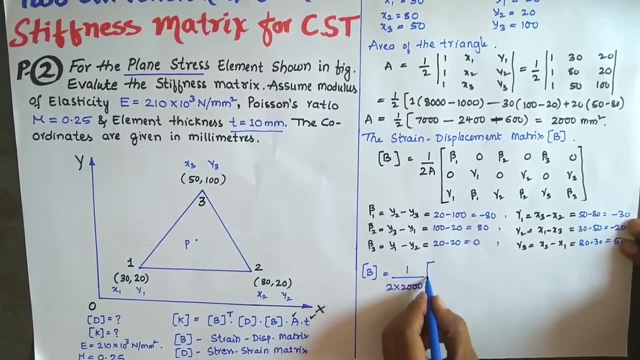 Now we will substitute in the B transpose, So in the B matrix, So 1 by 2A. A is 2000,. area of the triangular element: Again in the matrix So B, Beta 1 minus 80, 0.. 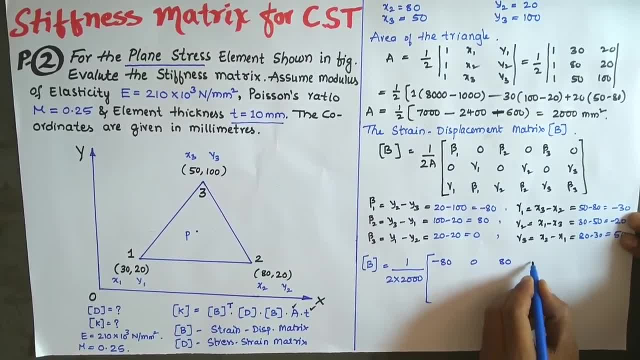 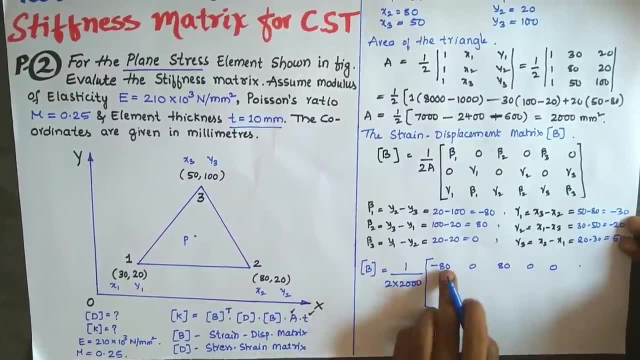 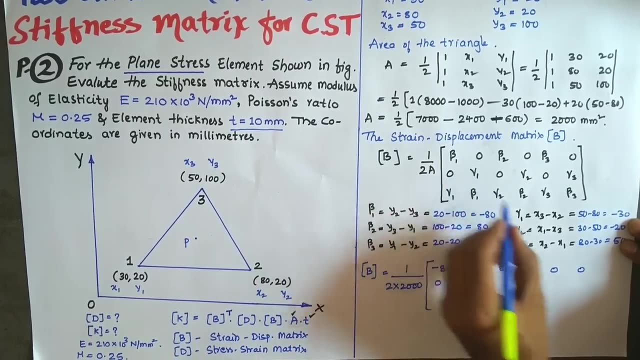 Beta 2, 80, 0.. Next beta: 3, 0.. Again, 0, last one, So 3, 0, B3, and 0.. Now 0,. gamma 1 is minus 30, 0.. 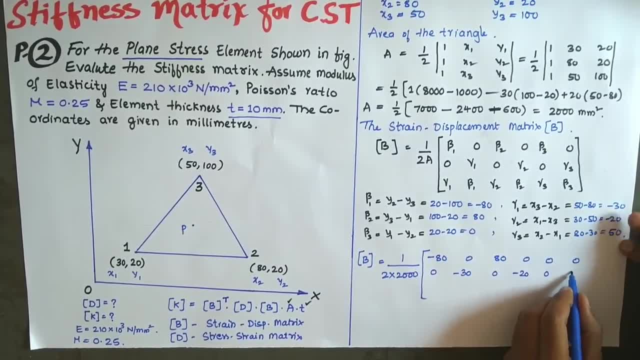 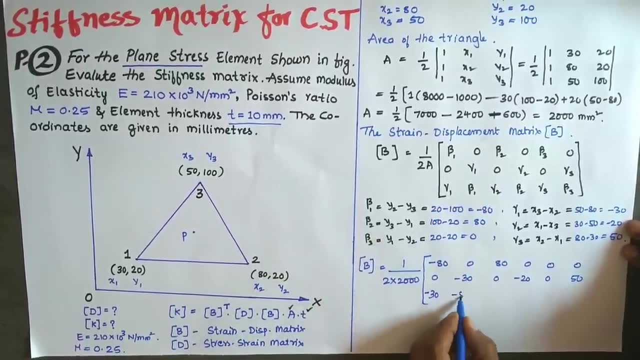 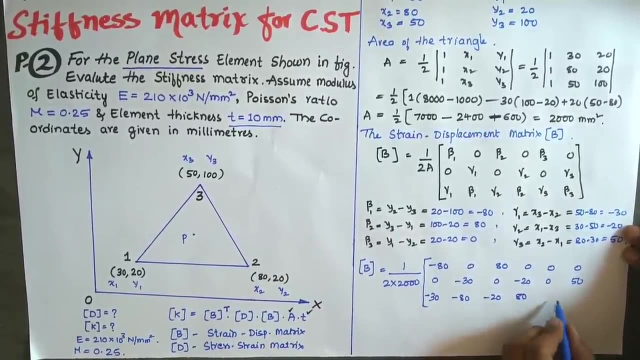 Gamma 2, minus 20,, 0.. Gamma 3, 50.. Next, gamma 1 is minus 30,. beta 1 is minus 80,. gamma 2, minus 20,, beta 2, 80, and gamma. 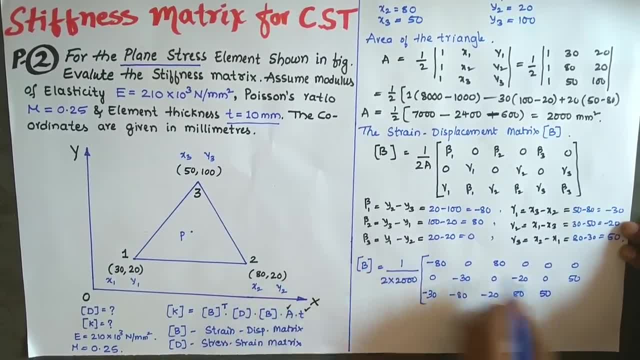 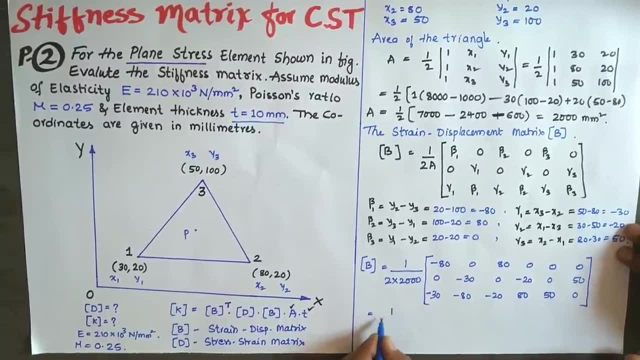 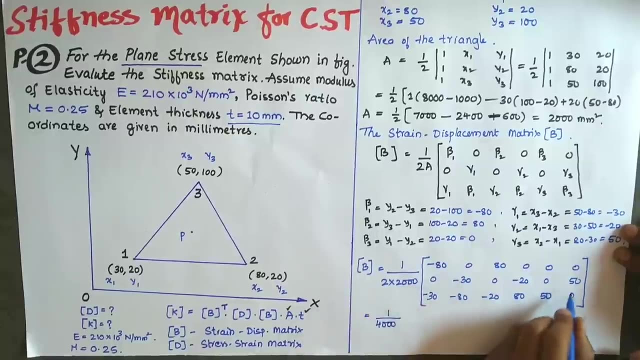 3 is 50, beta 3 is 0. So here, 1 by 4000.. Gamma 3, 0.. Gamma 3, 0.. So here, to reduce this step, we will take 10 outside to the matrix. 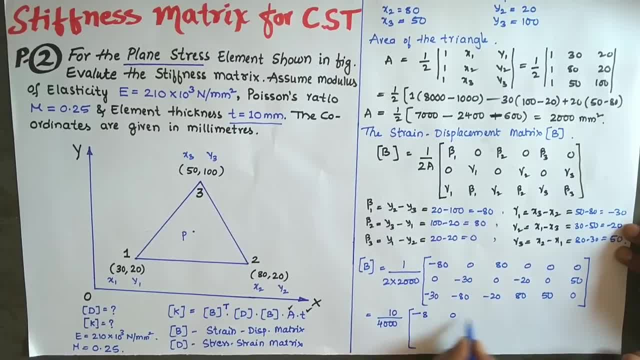 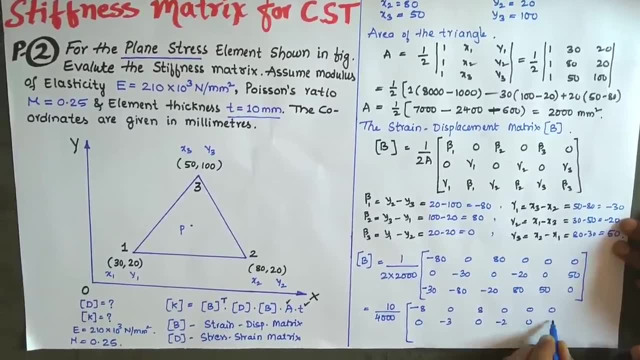 So inside we will have minus 8, 0, 8, 0, 0, 0.. So 0, minus 3, 0, minus 2, 0, 5.. Minus 3, minus 8, minus 2, 8, 5, 0. 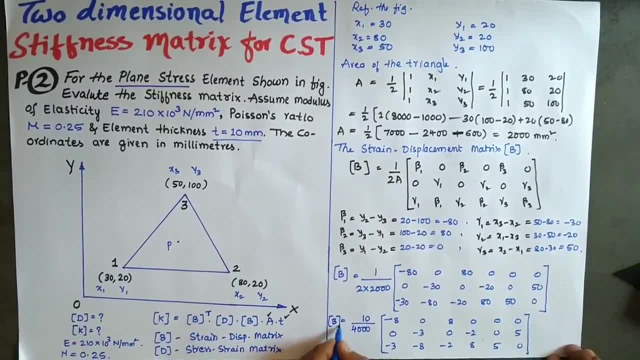 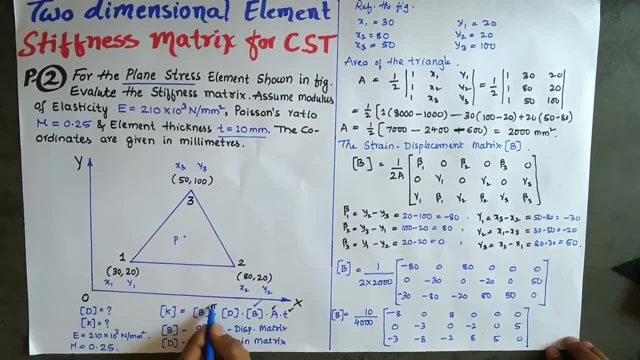 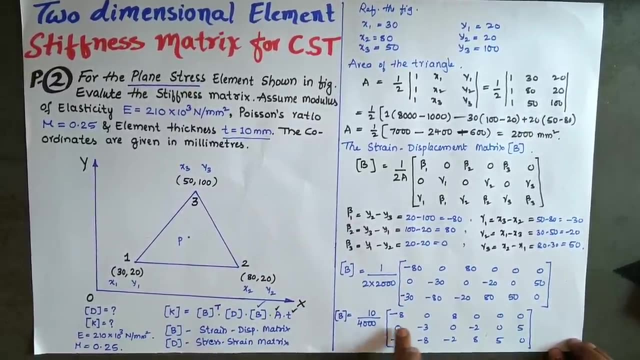 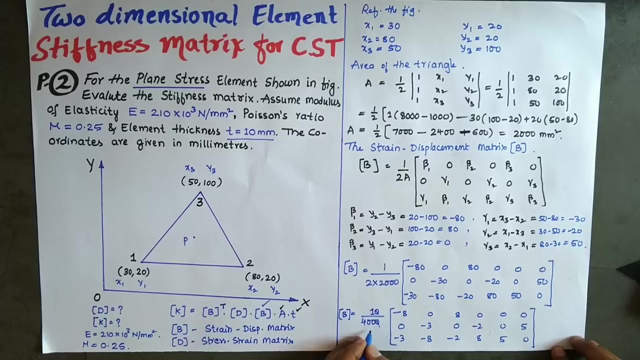 Okay, so this equation, it will be b matrix, that is strain and displacement matrix. so we obtain b. also now to calculate the b transpose. here, this row, it becomes an column in the b transpose, where this will be 1 by 400. so 1 by 400 again the row, it will be column in the b transpose matrix. 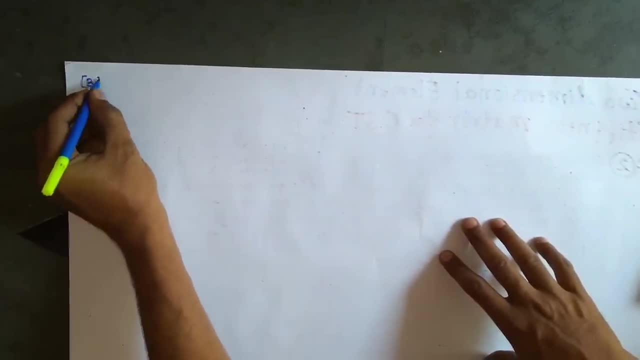 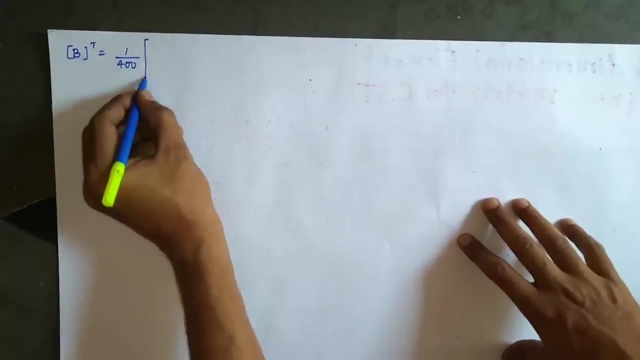 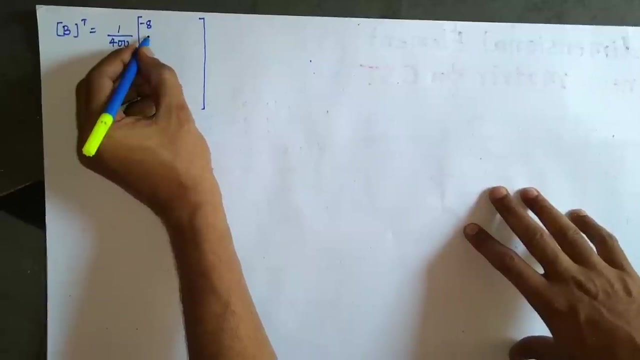 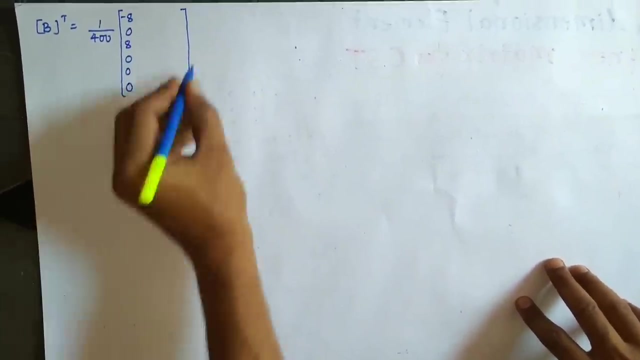 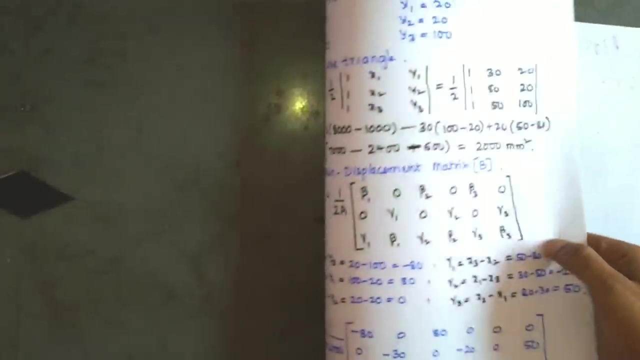 so we will calculate the b transpose now. so there outside it will be same as 1 by 400 again in the matrix. so minus 8, 0, 8, 0, 0, 0, 0. okay, so this is an a b transpose element. so we have calculated b matrix and now this is an b transpose element. 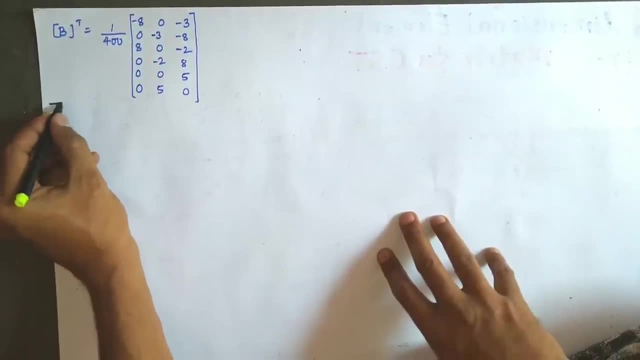 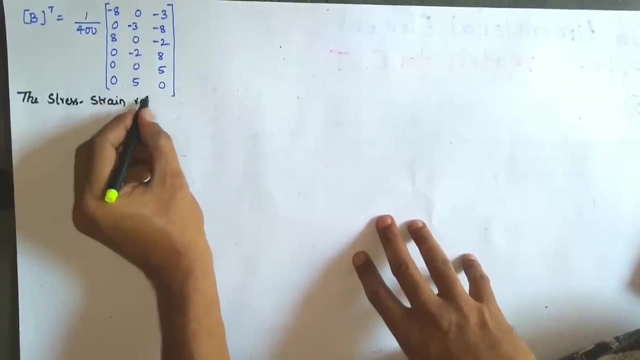 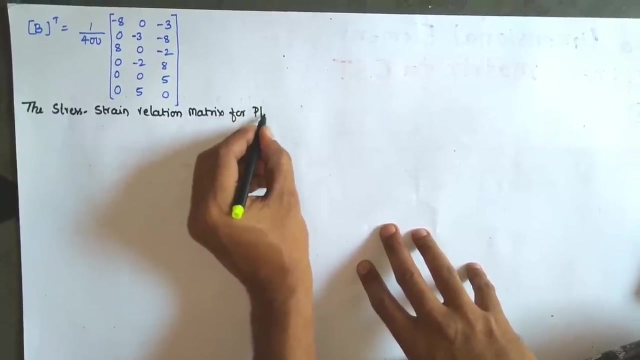 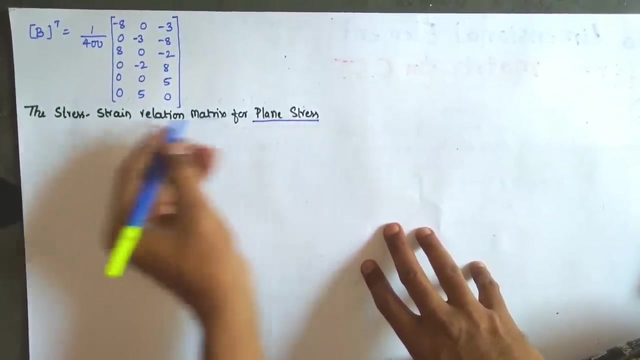 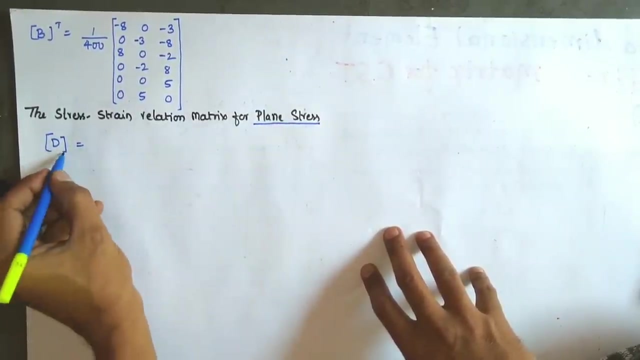 so after that we have to calculate the. the last one, the stress strain, relation, relation matrix for plane stress. so this point to be noted: here we are calculating for the plane stress. okay, for the plane stress. we are calculating for the plane stress, where it will be denoted with the capital d for both plane stress and plane strain. 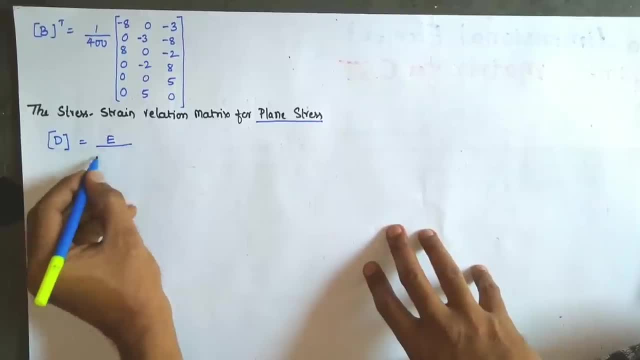 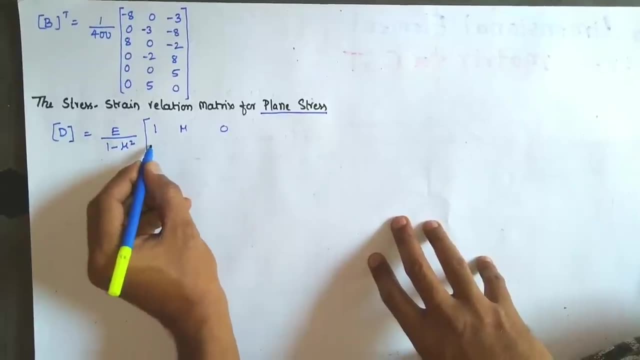 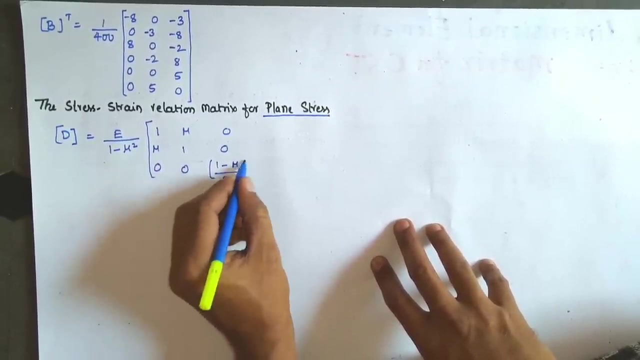 so where d is equal to e by 1 minus mu, square 1, mu 0, mu 1 0 0, 0, 1 minus mu by 2. okay, this equation is only for the plane stress, if the problem is related to plane stress. 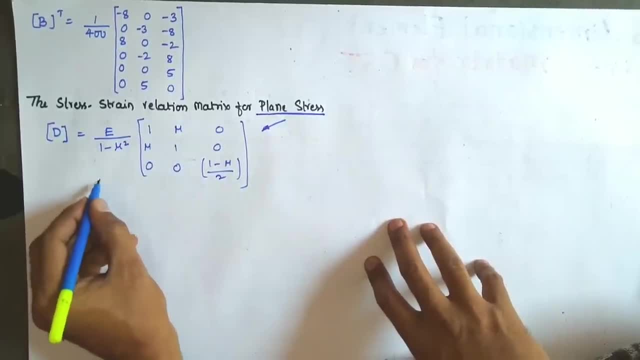 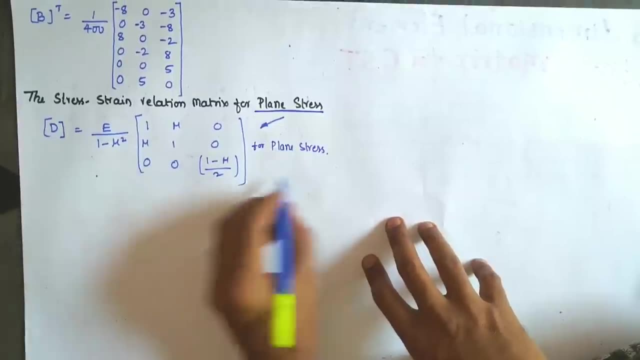 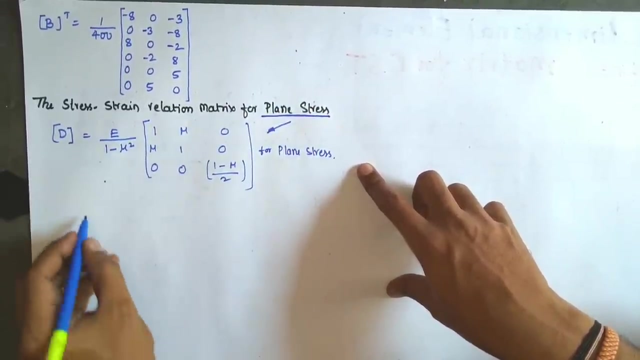 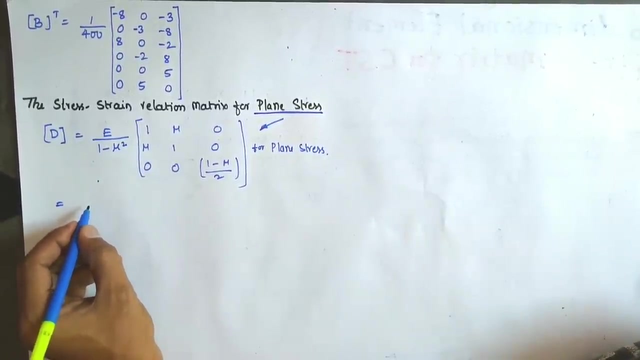 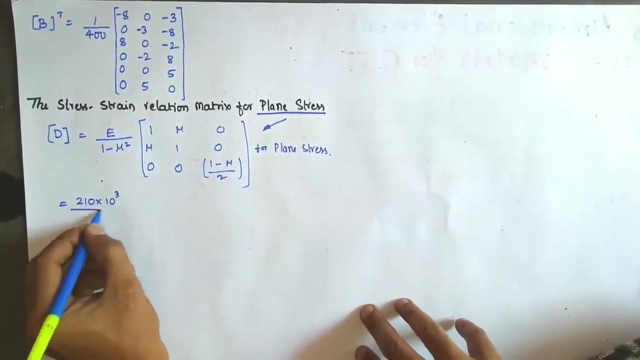 plane stress if you are having for plane stress. okay, so i will write the equation for plane stress, plane strain, later after completing this. okay. so value of e is given as 200, 10 into 10. power of 3 divided by 1 minus mu is the poisons ratio. that value is 0.25. 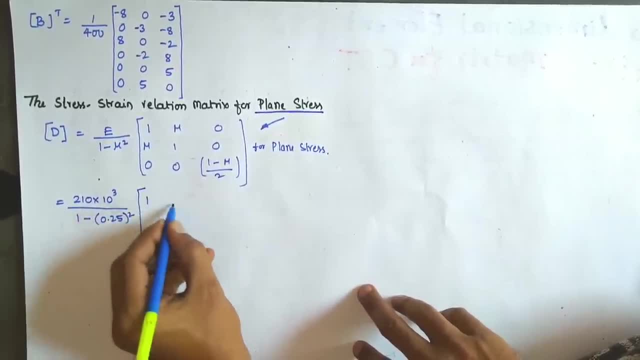 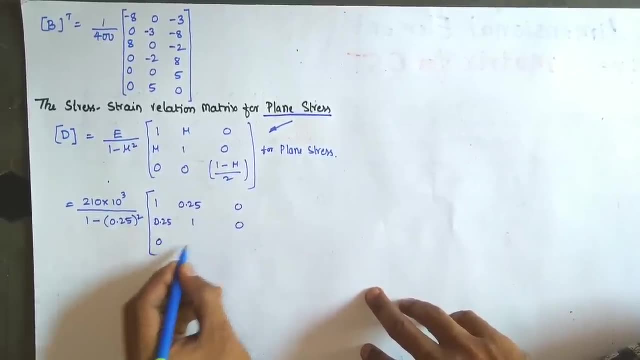 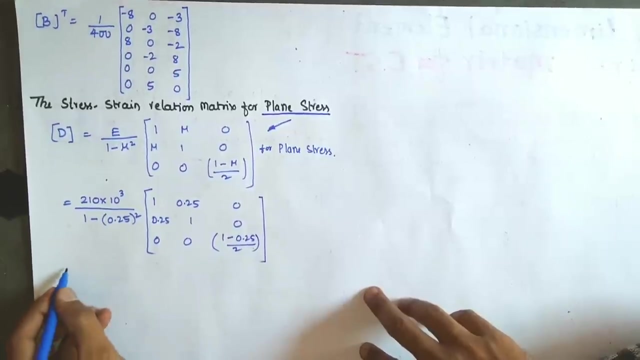 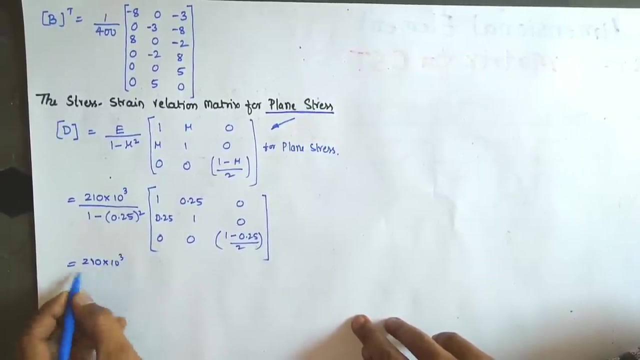 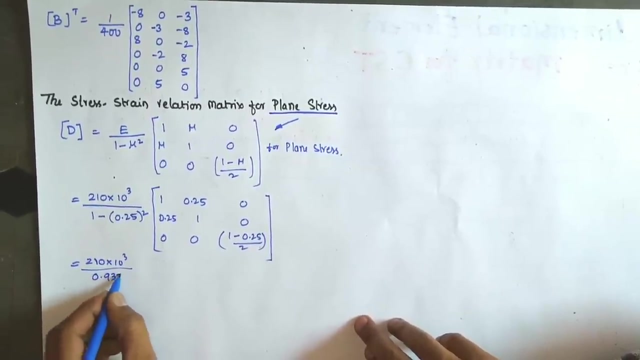 square again: 1, 0.25, 0, 0.25, 1, 0, so 0, 0, 1 minus 0.25 by 2, 10 into 10 power of 3. so here, after making the subtraction, we will get 0.93, 7, 5 again. 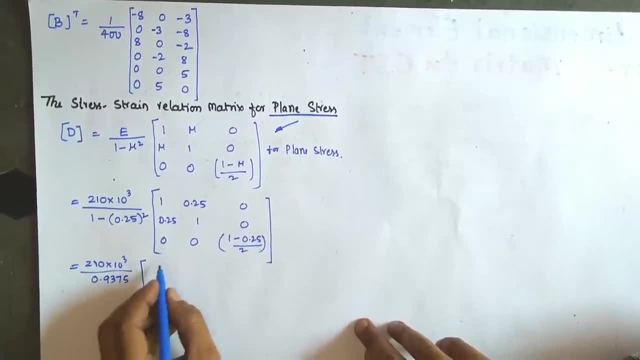 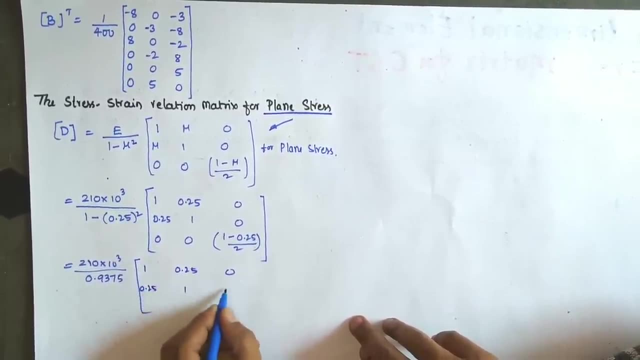 in the matrix 1 0.25 0, 0.25 1 0 0 0. so here after making the subtraction, we will get 0.93 7, 5 again in the matrix: 1 0.25 1 0 0 0. so 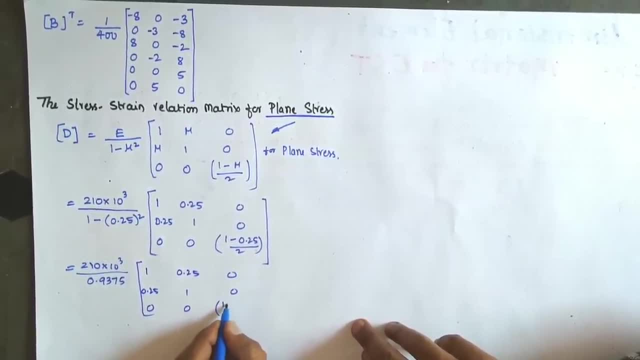 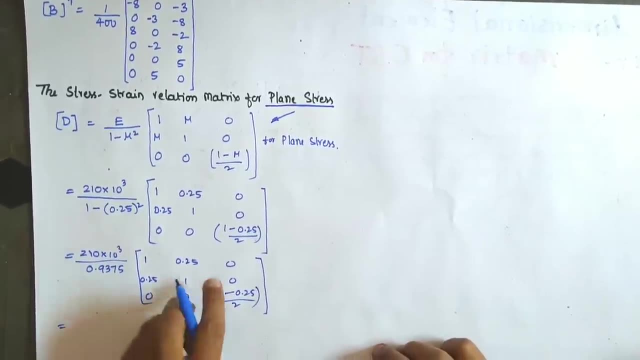 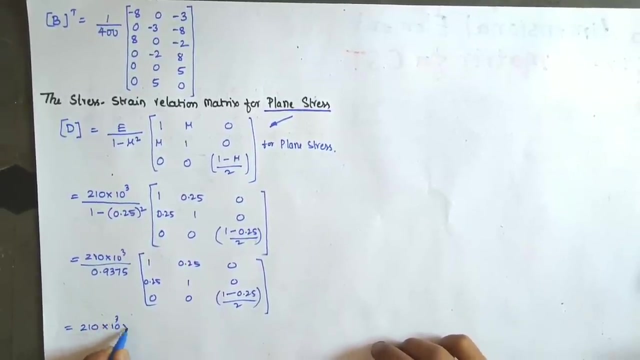 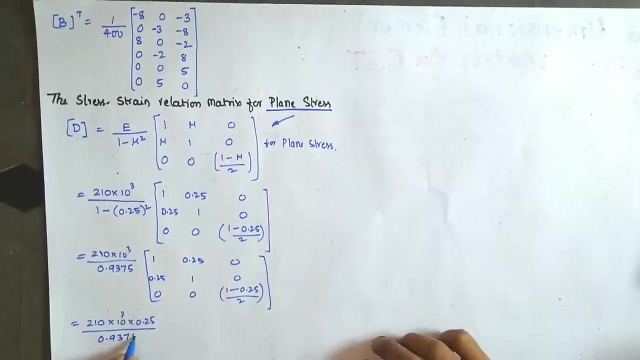 here one point zero, two, five by two. okay, so here we will make 0.25 outside the matrix. so 210 in 210, 4 of 3 into 0.25, divided by 0.93, 75, so 1 by 0.25, nothing. 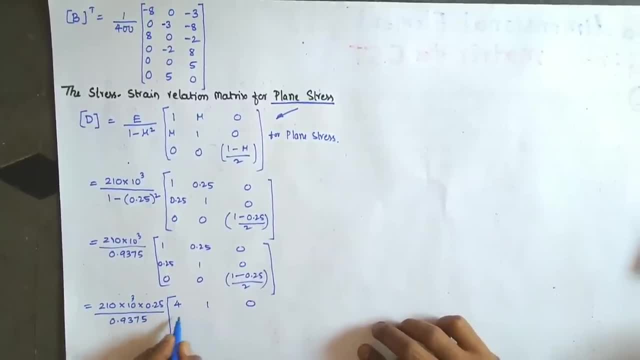 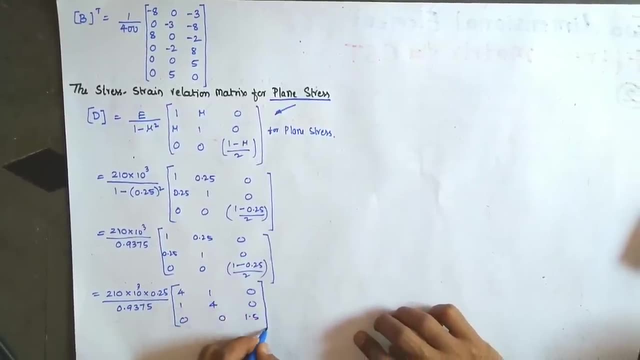 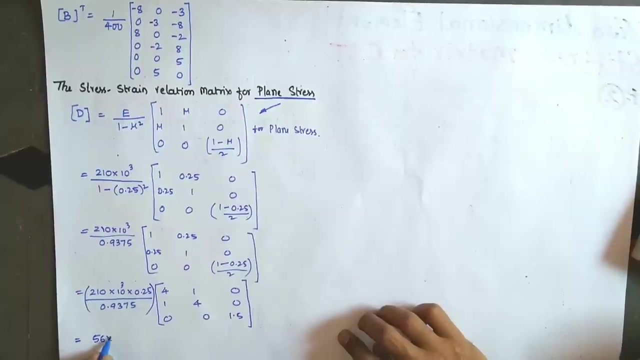 but it is in 4 1 0, 1, 4 0, 0, 0, 1.5. so this matrix you will get once you will take the 0.25 outside. so after making this calculation, we obtain 56 into 10 power. 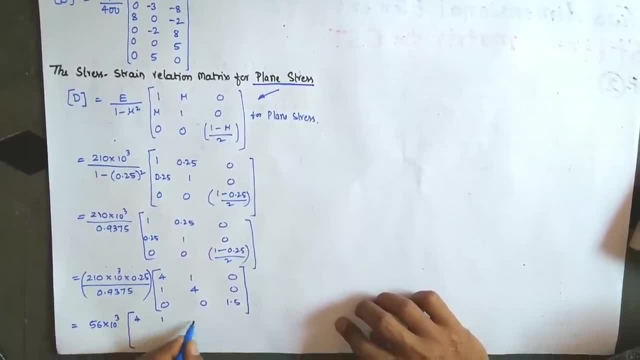 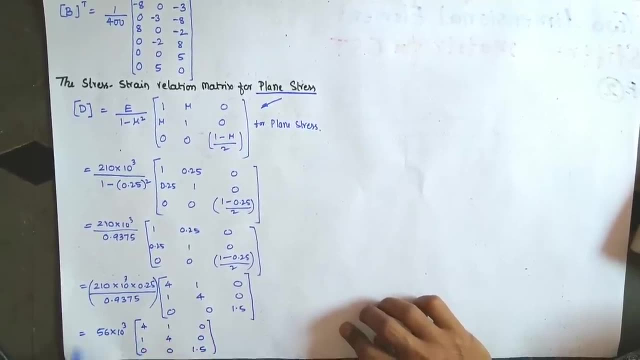 of 3. so again matrix 4 1 0, 1, 4, 0, 0, 0, 1.5. say this is equation 1.5. so again matrix 4 1 0, 1, 4, 0, 0, 1.5. say this is equation: 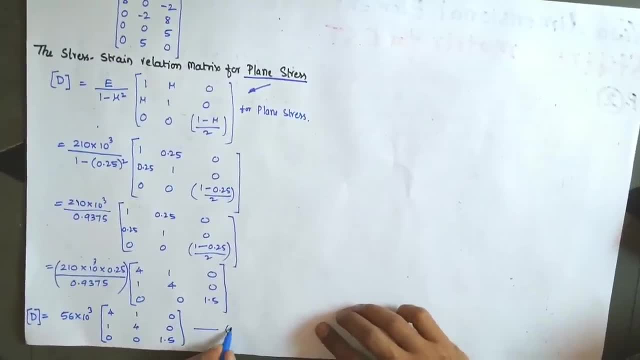 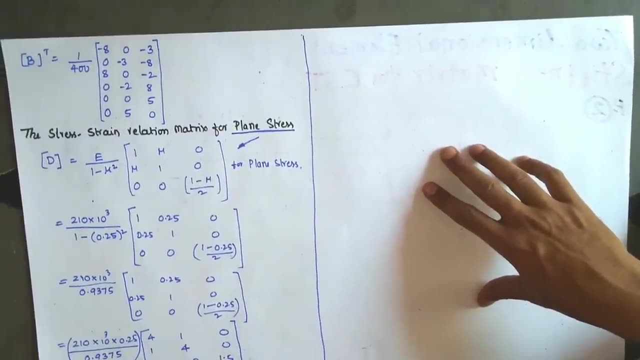 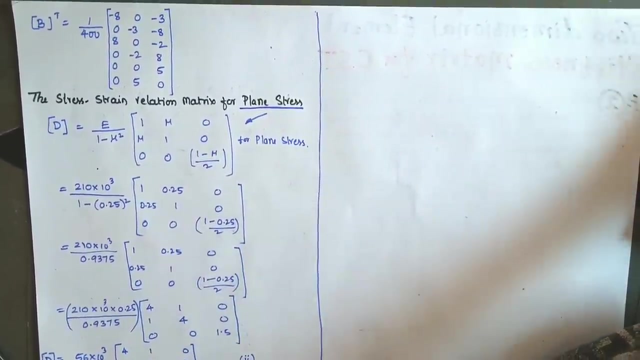 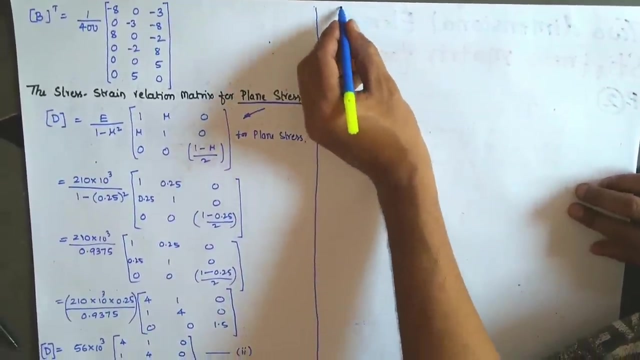 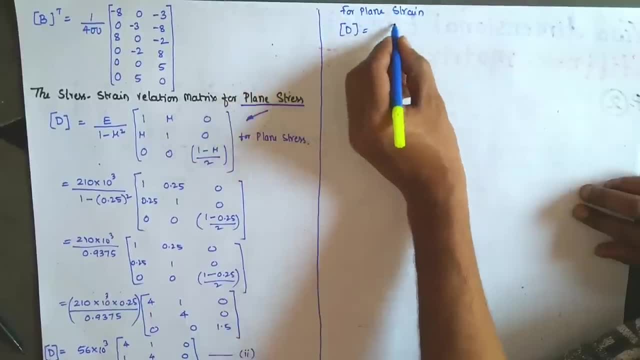 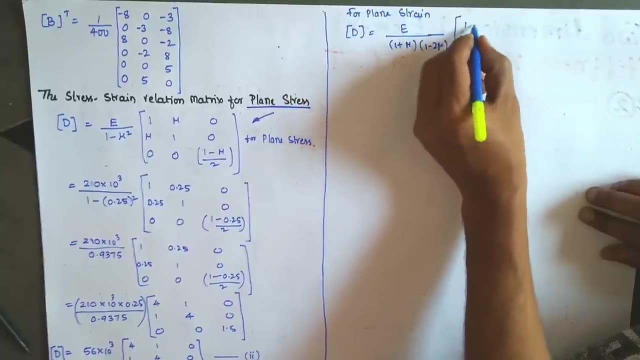 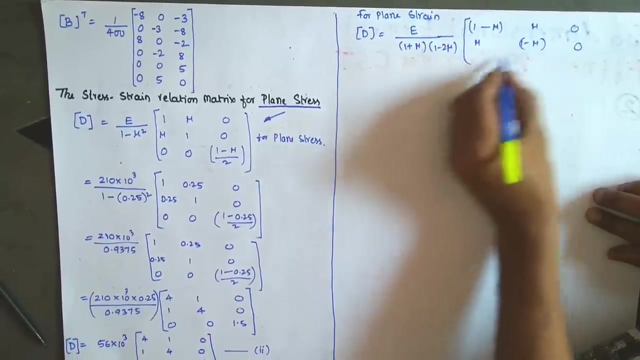 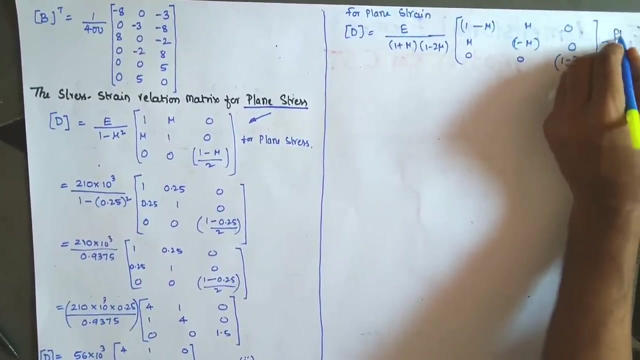 d is equal to e by 1 plus mu, 1 minus 2 mu, so 1 minus mu, mu, 0, so mu 1 minus mu, 0, 0, 0, 1 minus 2 mu by 2. so this equation you have to consider for plane strain elements. 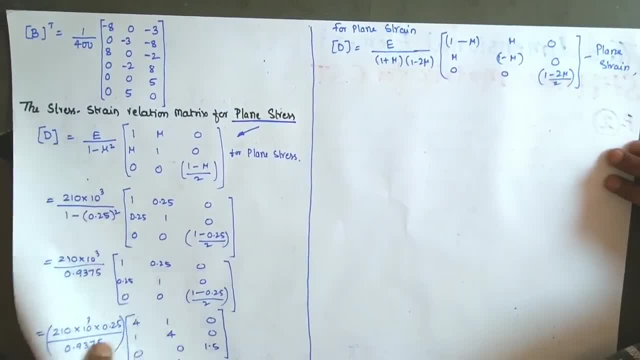 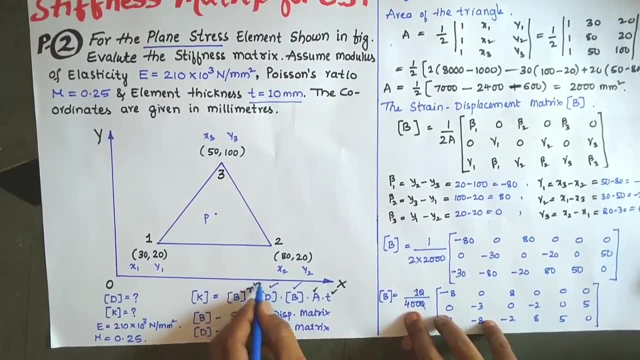 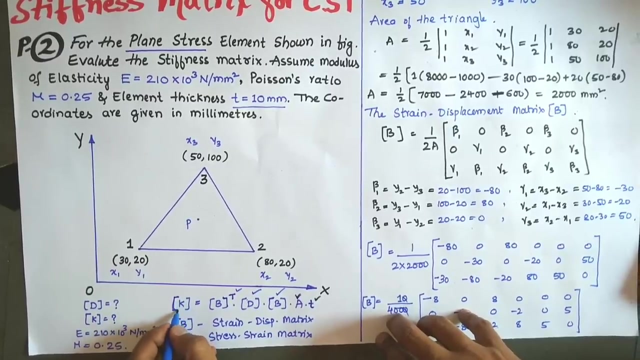 okay, so now we have finished all the values. so we calculated the b transpose d matrix. we have calculated and b also calculated. area is calculated and the thickness is calculated. after that we are going to calculate the stiffness matrix for the elements. so where k is equal to 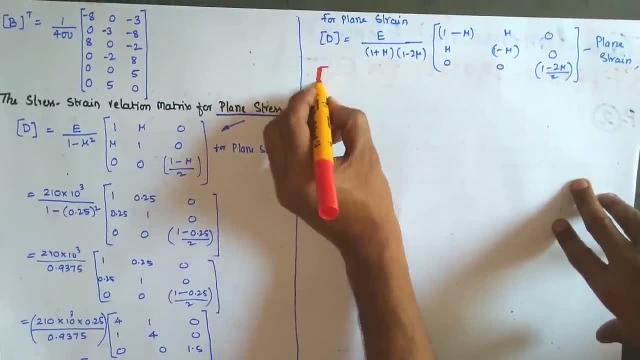 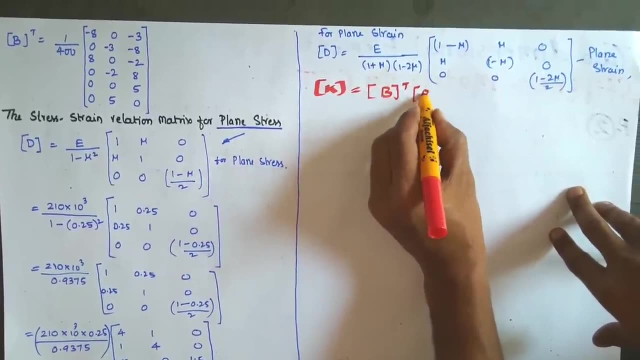 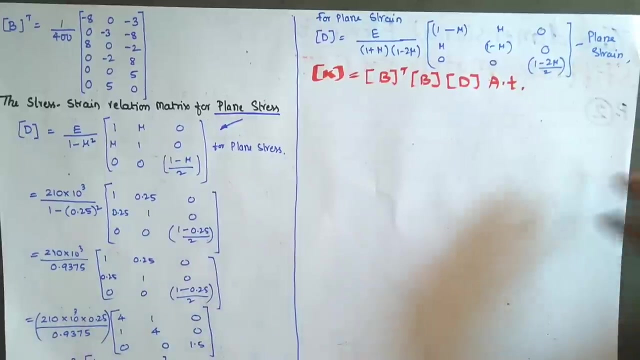 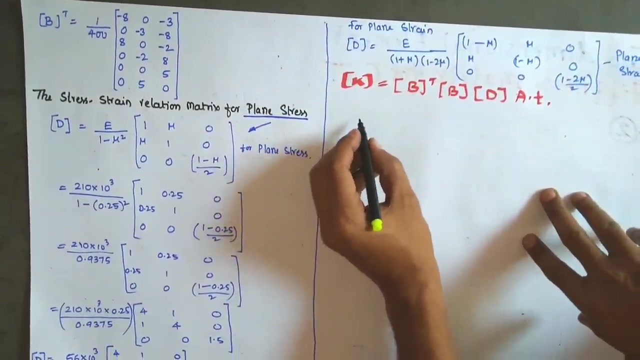 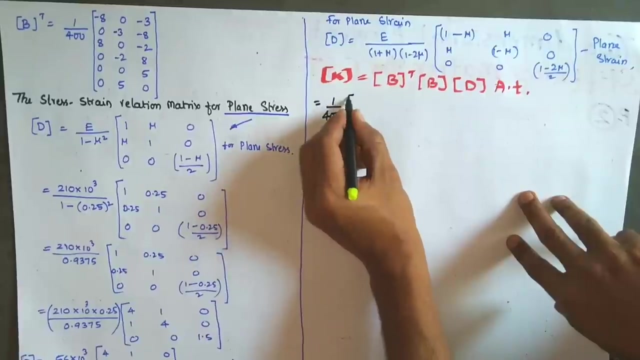 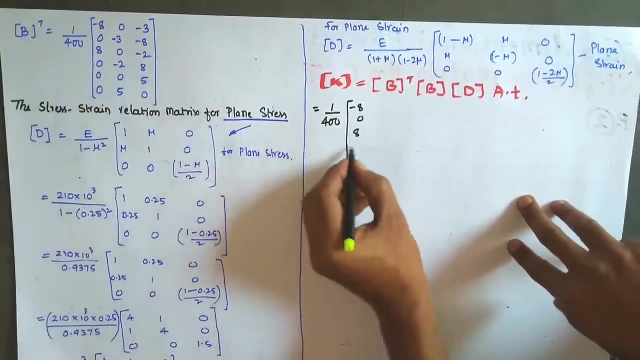 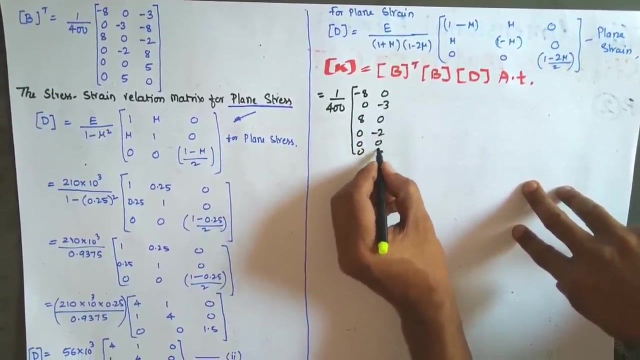 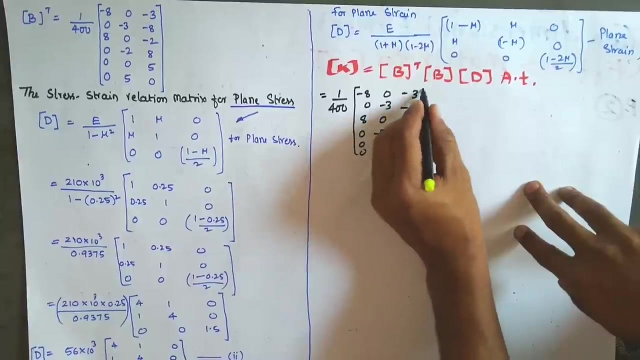 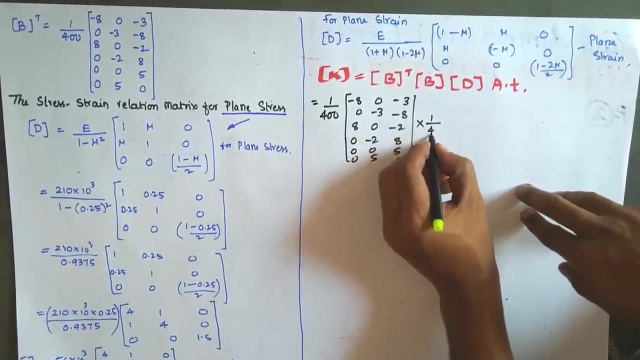 k is equal to it is b. transpose next b, again d, then a into t, so write all the equation now. so for the b transpose 1 by 400 minus, such that c. so let's give acieru equation now, because if we use after statement that foot is minus. 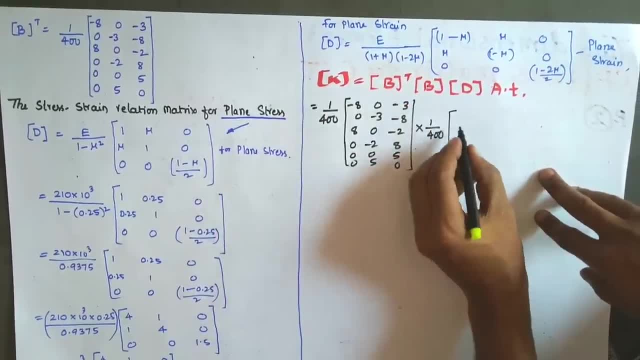 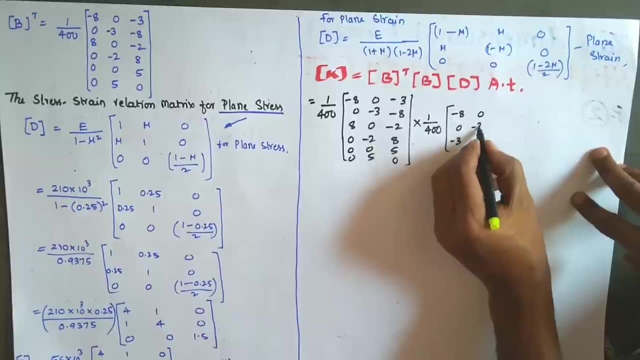 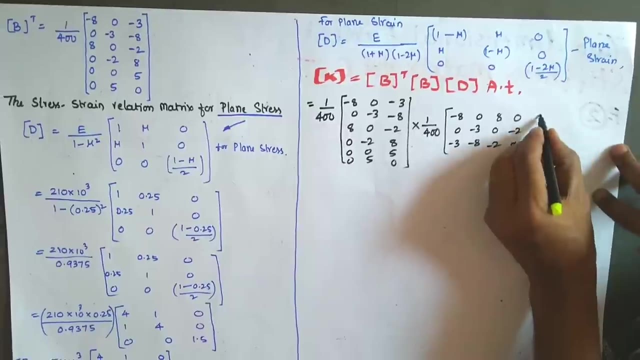 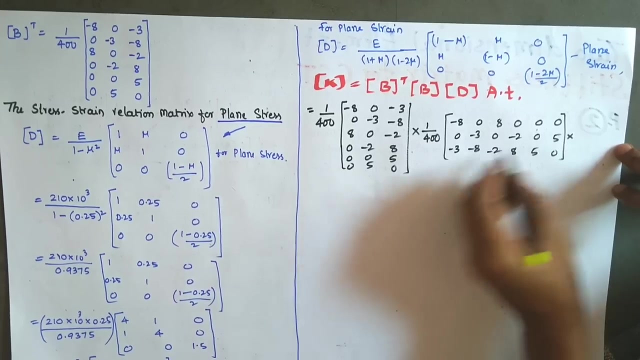 here this row, it becomes n column. so minus 8 0 minus 3, 0, minus 3 minus 8, 8 0 minus 2 0 minus 2, 8 0 0, 5 0, 5 0 into next the D transpose for the D matrix we. 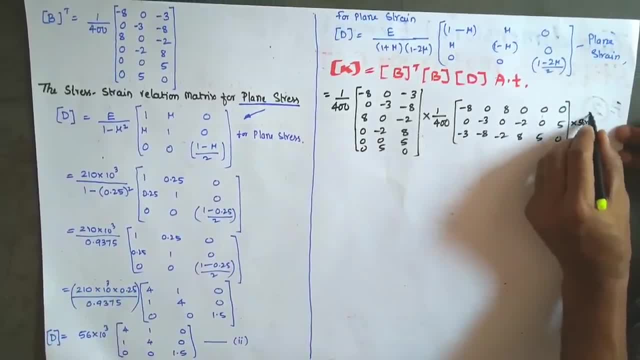 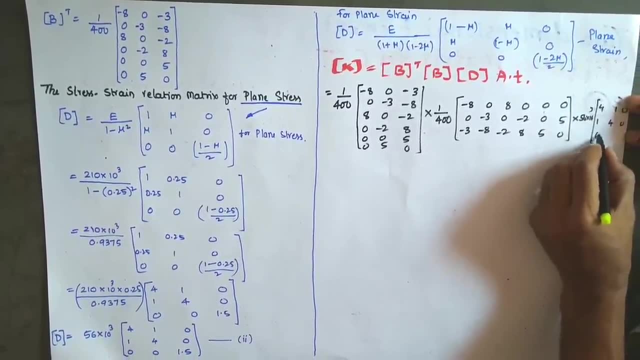 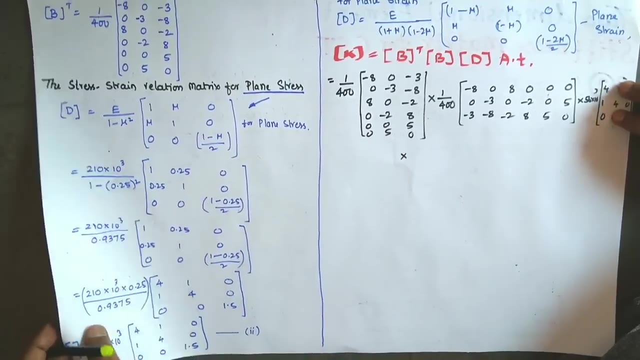 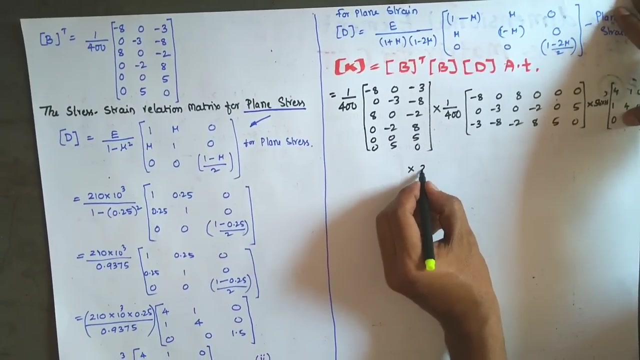 got as 56 into 10 power of 3. again matrix 4 1 0, 1, 4 0 0 0, 1, point 5. so into the area of the element. so area of the element is 2,000 into the thickness. 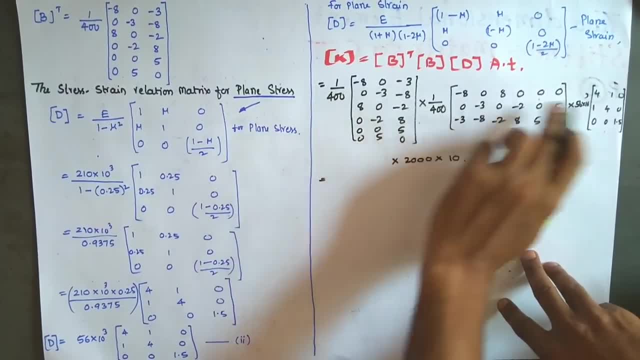 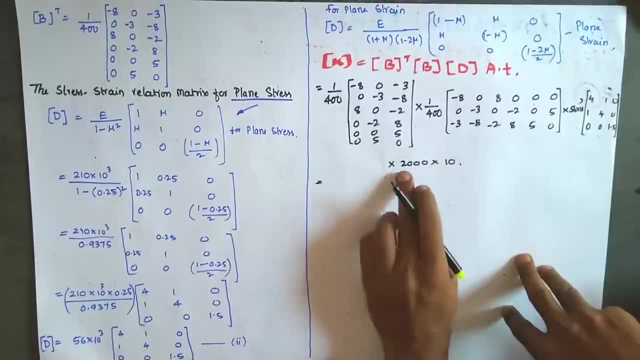 is 10 m. okay, now what do we do? whatever the outside value is there, you make the multiplication that is 1 by 400, 1 by 400 into 56 into 10, power of 3 into 2,000 into 10. so after making this, we will have 56 into. 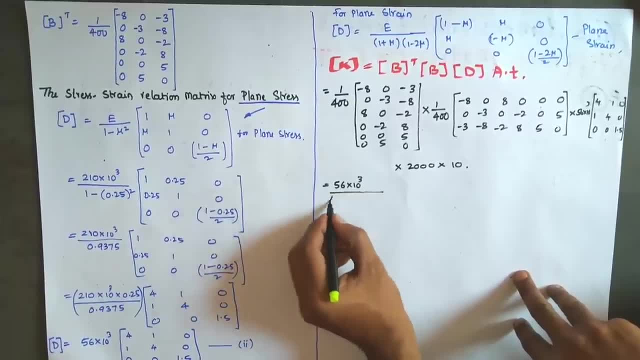 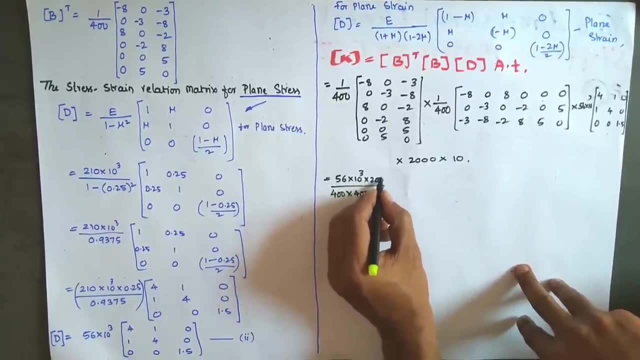 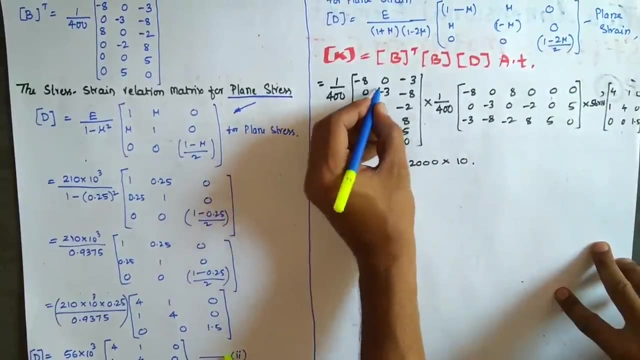 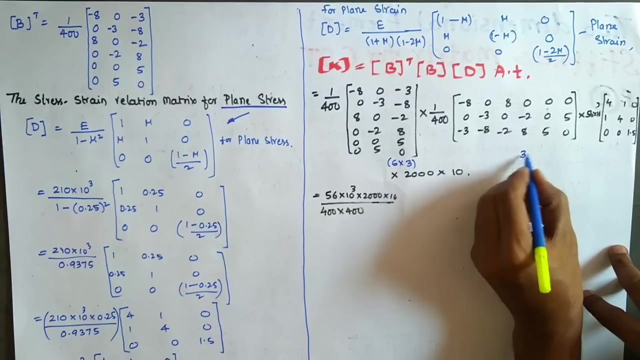 10, power of 3 divided by 400 into 400. so again here, 2,000 into 10. so this will be the outside the matrix- tell me that variable is somewhere- is a matrix because earlier this region was so declared very important but still today it is so declared. so here this matrix is. 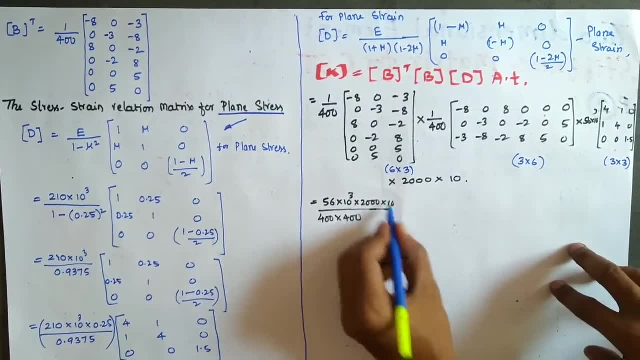 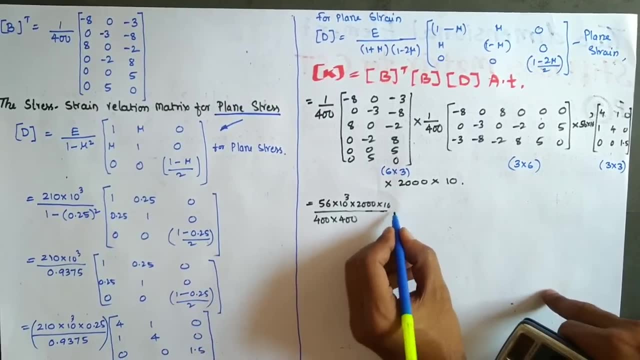 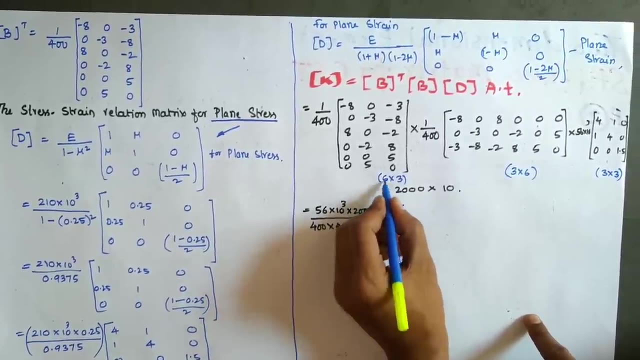 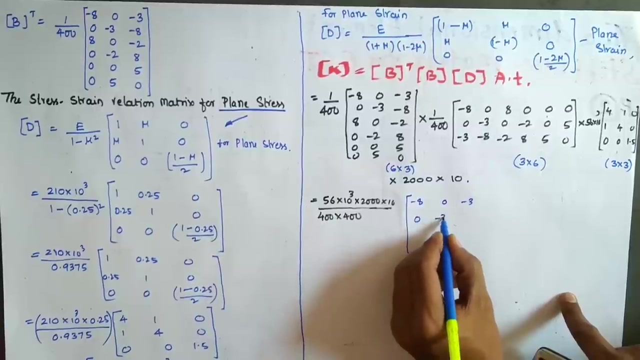 n 6 into 3 matrix and the second one is 3 into 6 matrix. again, the last one is 3 into 3 matrix. okay, so we have considered all the values outside. so here, if we make this calculation, we will get into 3 into 3. so minus 8, 0 minus 3, 0 minus 3, minus 8, 8, 0 minus 2, 0 minus 2. 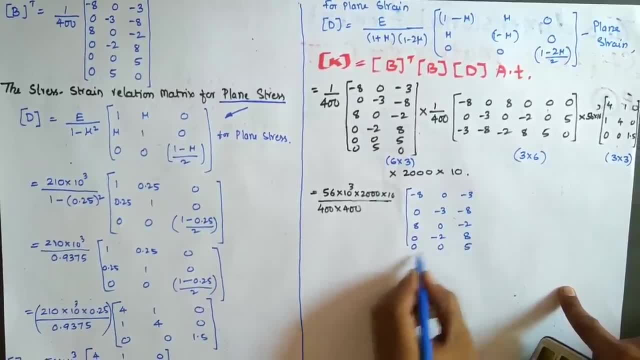 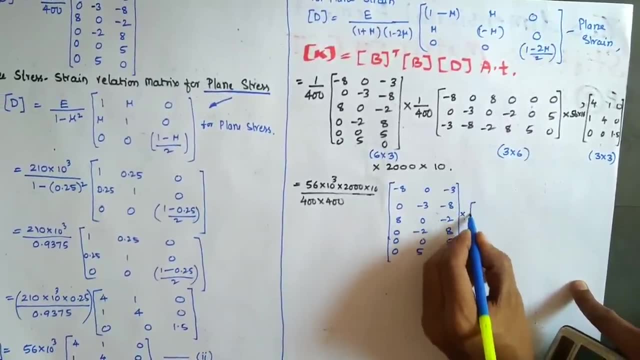 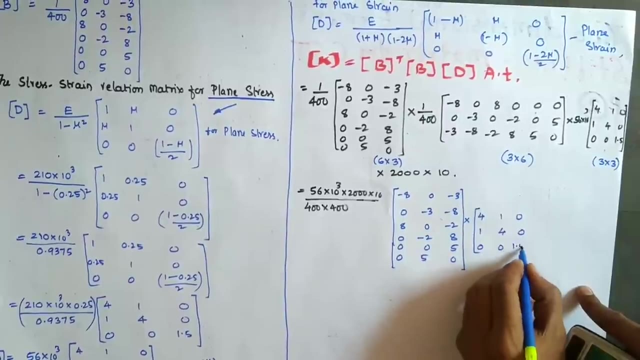 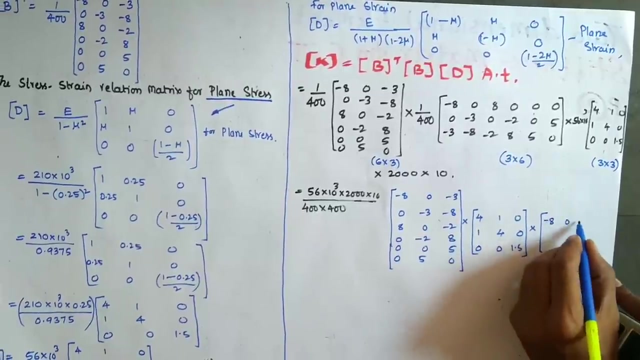 8 0 0, 5 0, 5 0. into this 3 into 3 matrix: 4 1 0 1, 4 0 0 0, 1 point 5. so into the 3 into 6 matrix you have to write 8 0, 8 0 0 0 0 minus 3 0 minus 2 0 5. 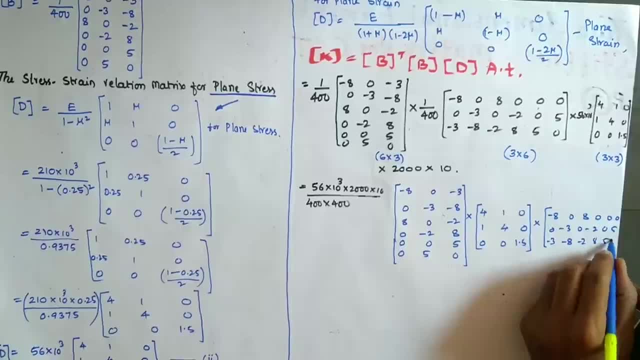 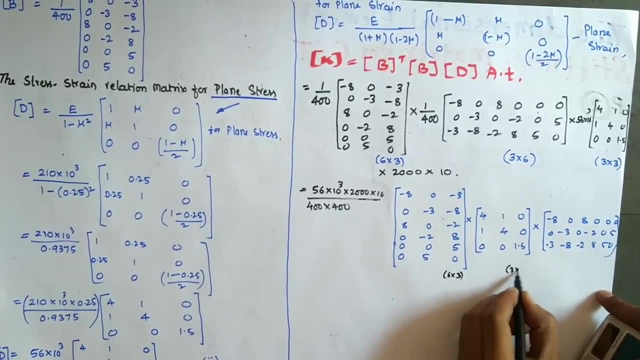 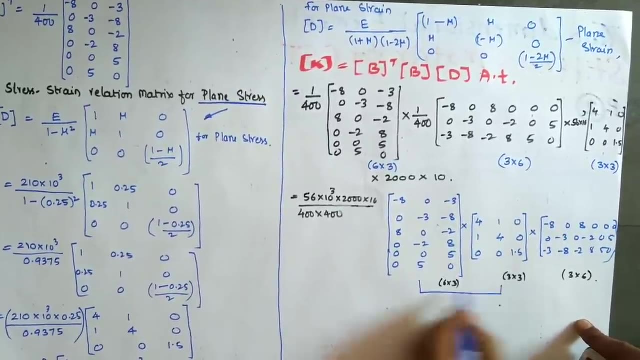 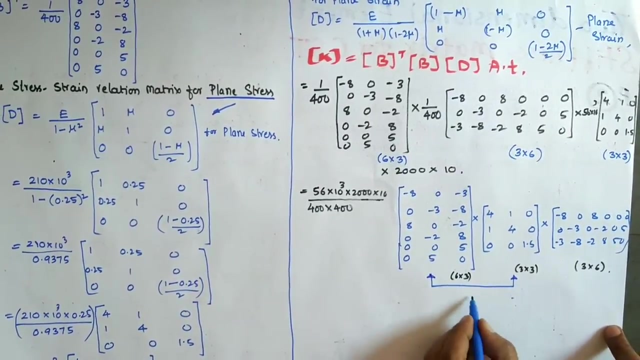 minus 3 minus 8, minus 2, 8, 5, 0. so here now it is 6 into 3, 3 into 3, 3 into 6. okay, so first we will make the multiplication of these two, then after that, whatever will obtain, we will obtain the. 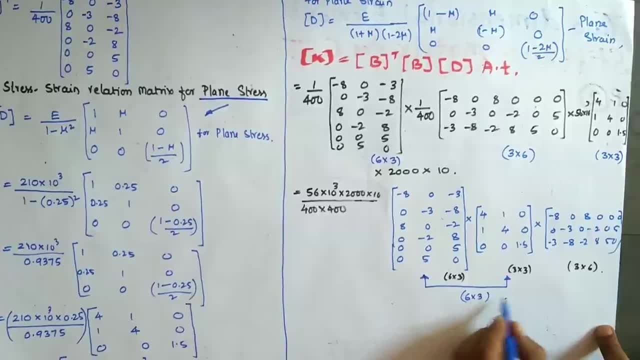 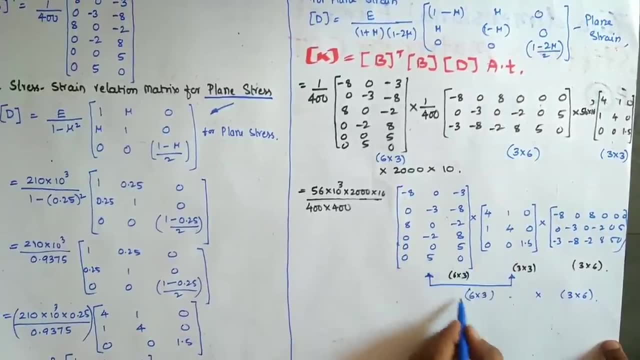 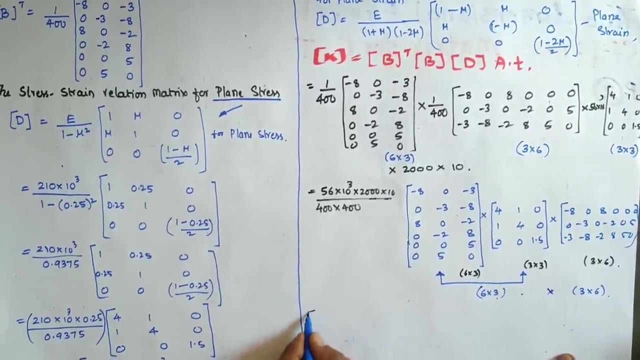 matrix, like 6 into 3 matrix, will opt it. so this into 3 into 6 matrix. we have to make the multiplication. okay, so from these two will get 6 into 3. into this, 3 into 6, you have to make the multiplication. so after making the multiplication we will write the direct answer. so here after this: 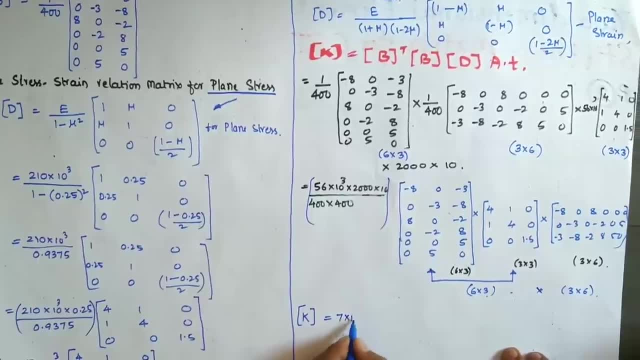 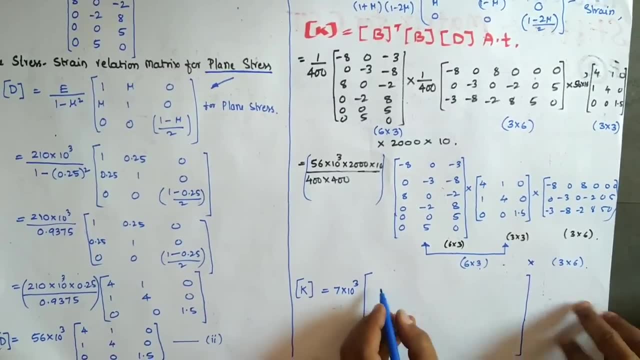 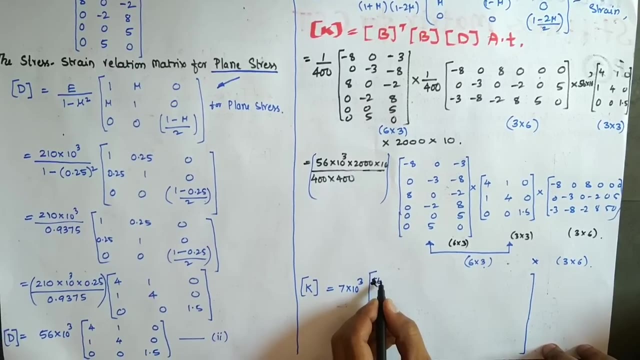 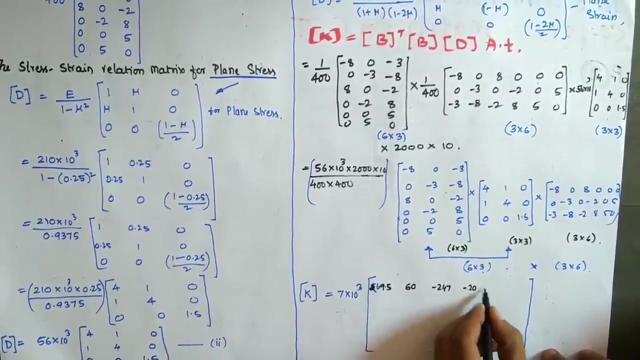 calculation, I obtained 7 into 10 power of 3 as the outside value, so now we will get the multiplication. so after this calculation, I obtained 7 into 10, power of 3 as the outside value. so now inside the matrix 5, 16- sorry, it's 269 point 5- 60 minus 247 minus 20 minus 22. 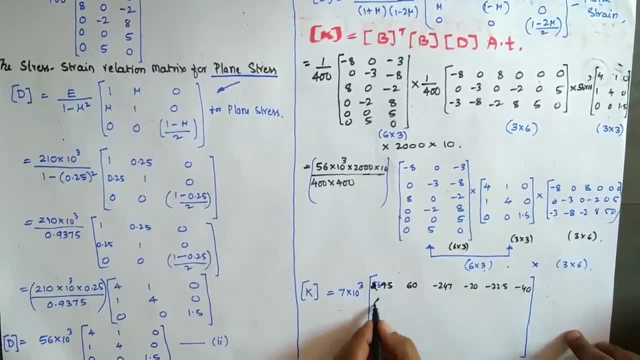 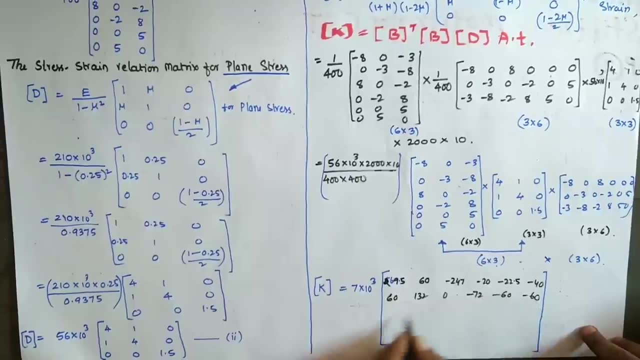 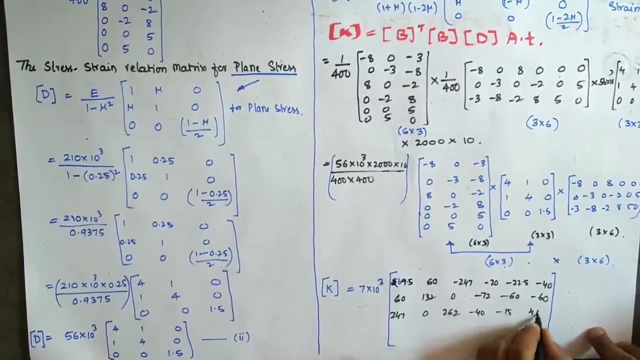 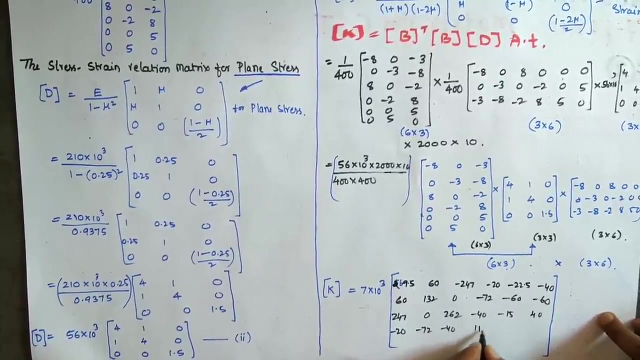 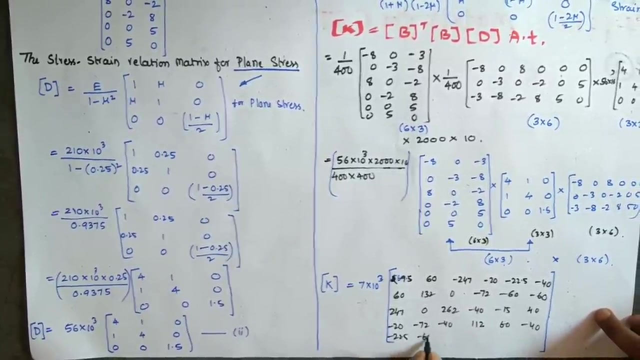 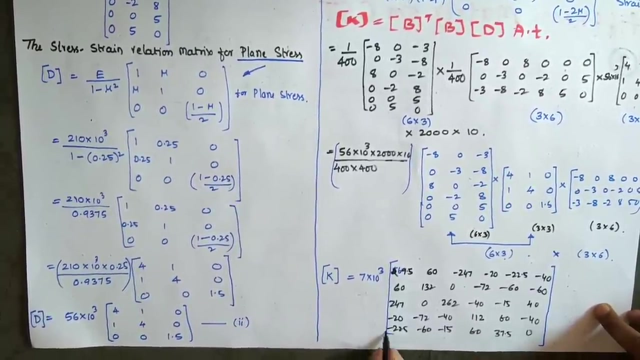 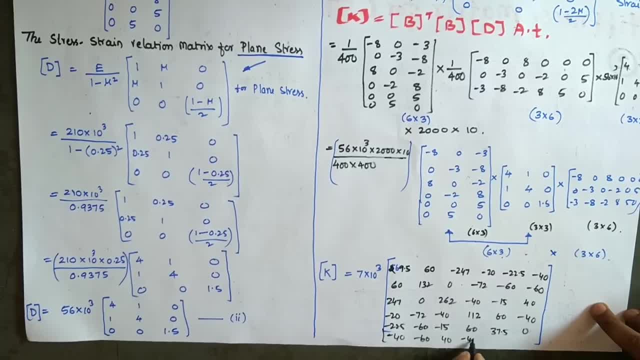 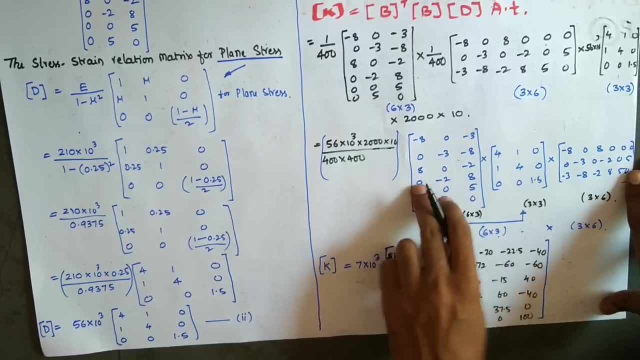 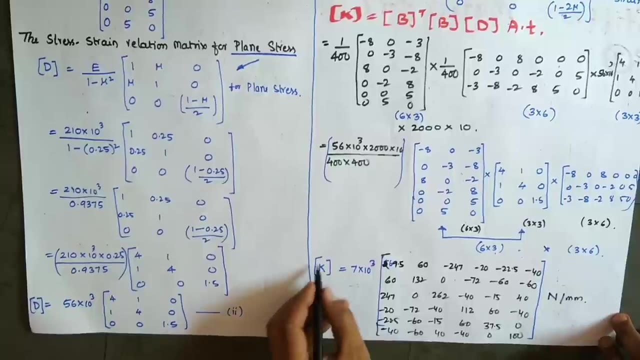 60, 40 minus 40, 0, 100. so this is a equation you will obtain by multiplication of all the three elements. okay, the unit of the stiffness matrix, it will be newton per millimeter. okay, so we have calculated the stiffness matrix for the a triangular element.